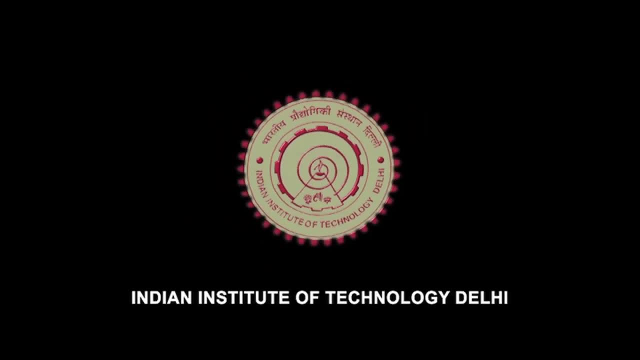 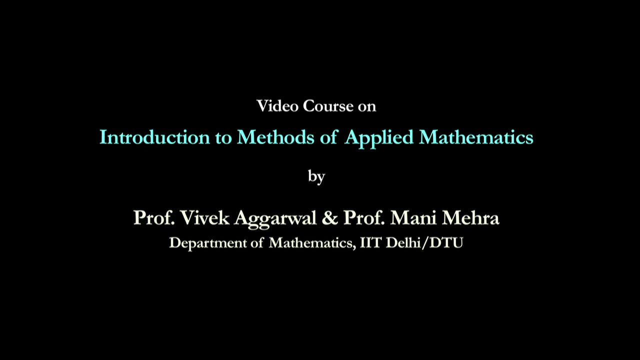 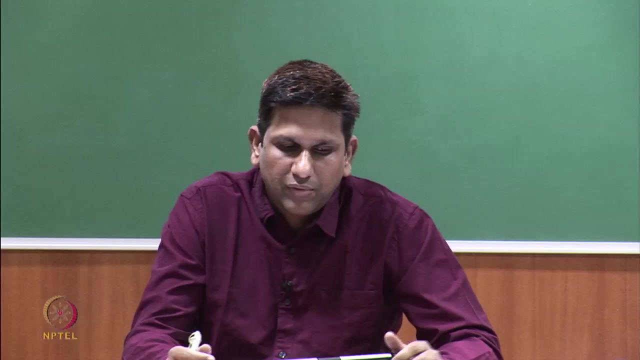 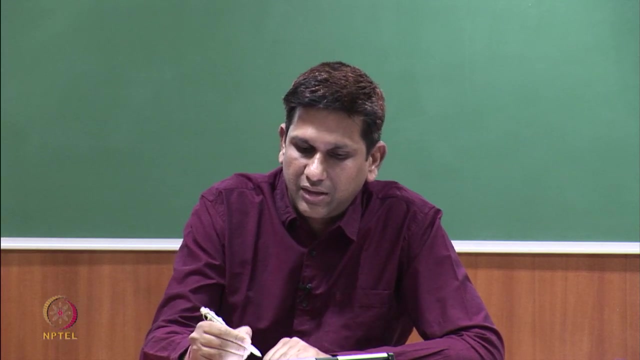 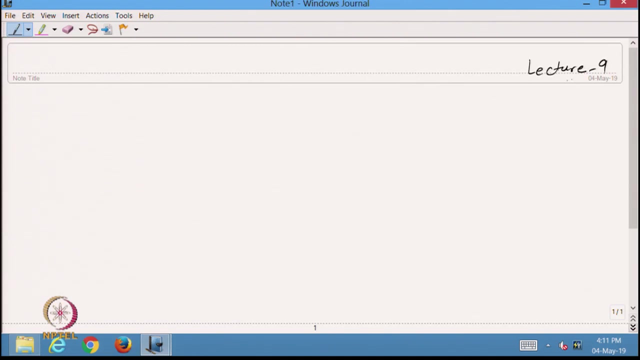 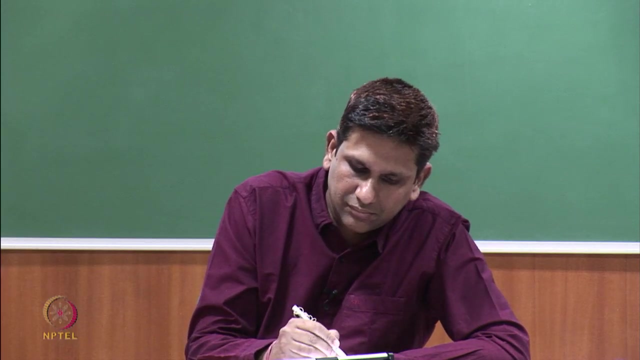 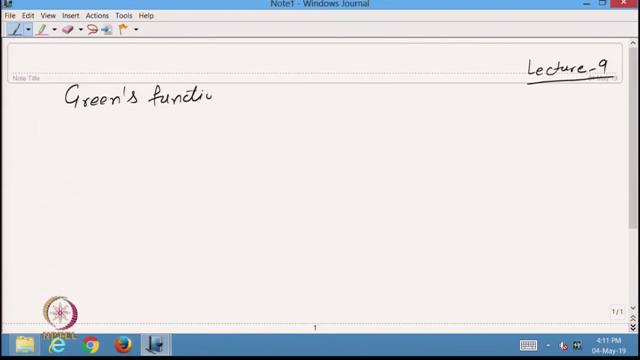 Welcome viewers back to this course. So today we are going to discuss the lecture 9.. So today we are going to start with a new topic and that is called Green's function. So this Green function is basically used to find out the 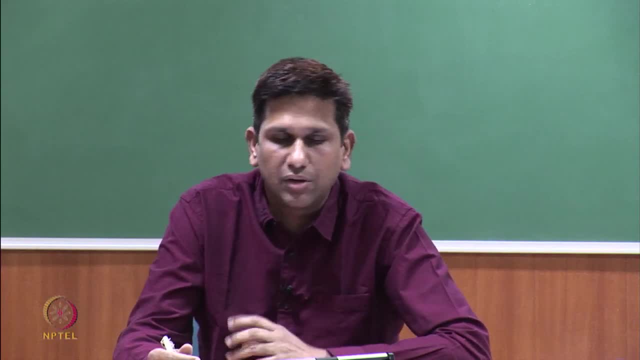 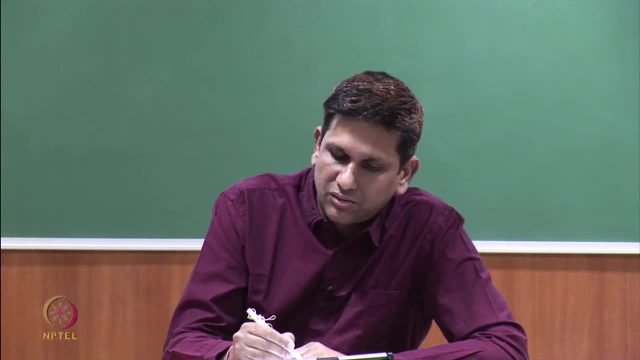 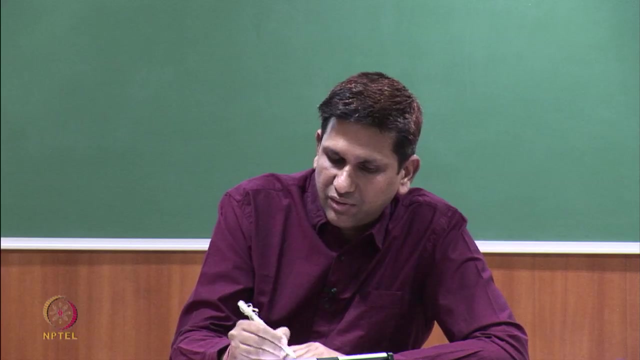 particular solution of any second order or any linear differential equation. So as we have been doing this course, so in the last class also, we have started with second order differential equation. So L is my differential operator and this is the differential operator. 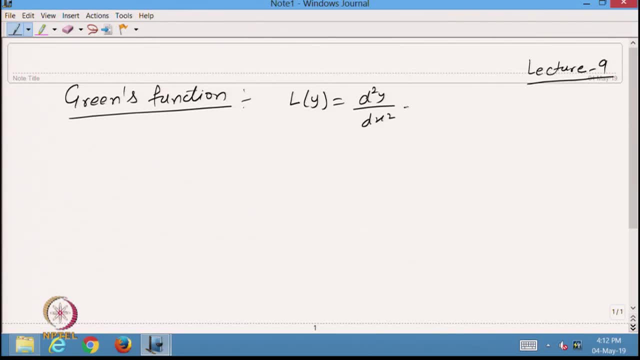 we have defined d square y over dx square plus p x dy, by dx plus q, x, y equal to f x. So this equation- I know that this can also be written as L of y, because y is a function of x, So we can also write this equation as p x y dash- 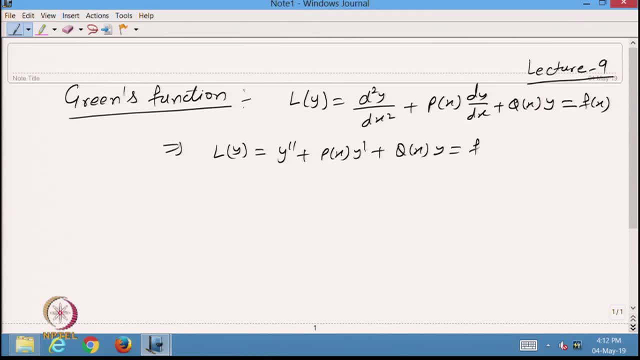 x plus q x, y is equal to f x. So in this case we are taking the boundary domain, So x belongs to the interval, that is, a, b, the closed interval, and we are assuming that the p, x and q x and f x, all are continuous. 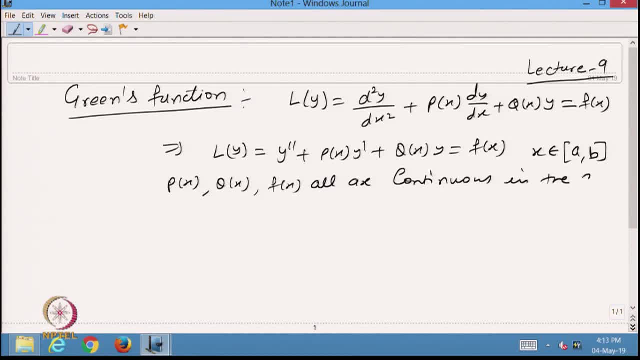 in the given domain. So now is this differential equation. I call it equation number 1.. So this equation I can write as a L y operating on a y is equal to f x, And if I want to solve this equation, I take the solution y x and I take L inverse f x, where this L inverse 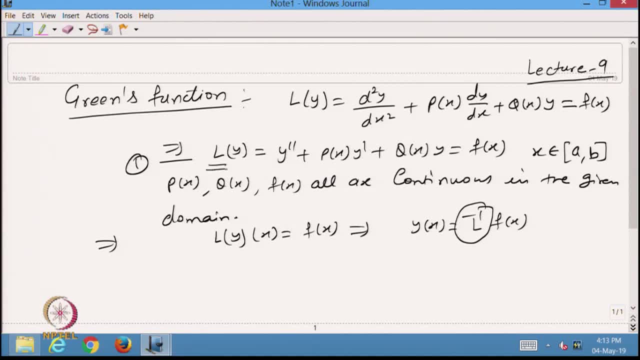 because it is the. I know that the L is a differential operator, So this inverse will be the integral operator. So this integral operator is called integral operator Green's operator. So this is the inverse of the given differential operator. So now, 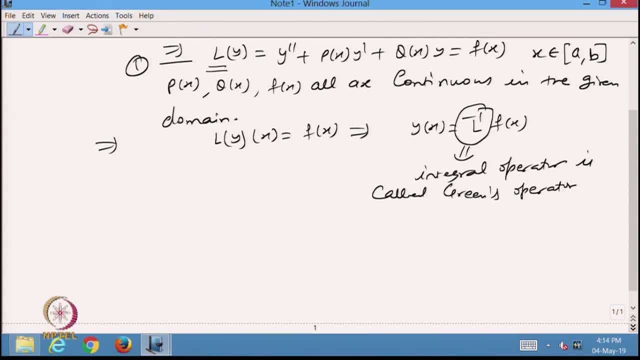 we are means we are dealing with the linear second order, homogeneous linear second order, differential equation, So this L inverse. So because if I am able to find this L inverse, then I can find the solution of this equation And then we are able to solve the differential equation because. so, if you see this one, 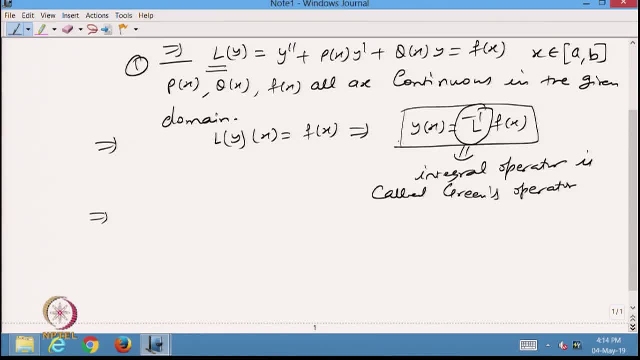 in this case, I am solving this equation. So basically what I am going to do is that this, my y, x, will be a particular solution, Because we are solving the differential equation, that is, a known homogeneous equation, And for that we know that, whatever the solution, 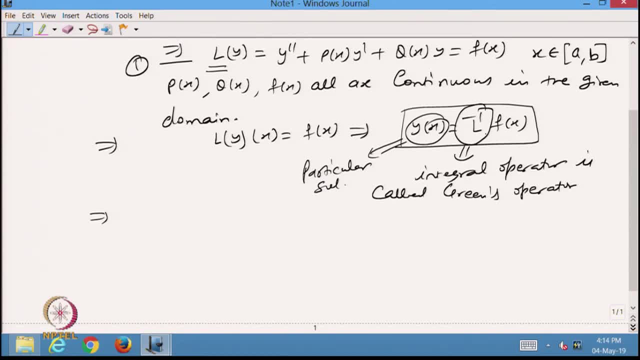 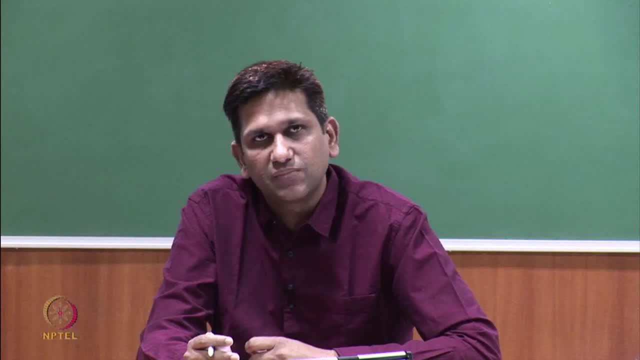 comes, that is called a particular solution. So this equation is true. Next I will cross the two over some merges. whereas first one We already know the different methods when my function, fx, is some exponential function or a sin cos function or some other function, but we have solved this one when the given 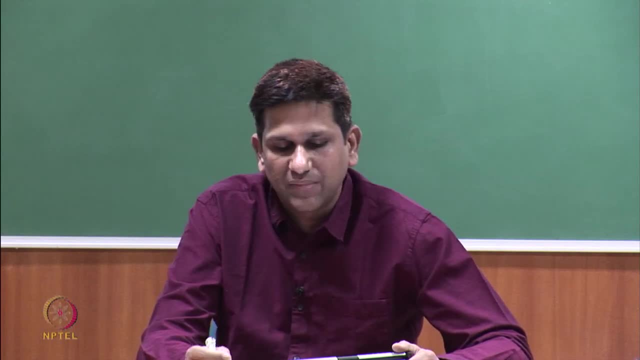 differential equation has the constant coefficients And after solving the constant coefficient homogeneous equation, we are able to find the complementary solution and based on the type of the function- fx on the right hand side- we can apply the different methods to find out the particular solution. 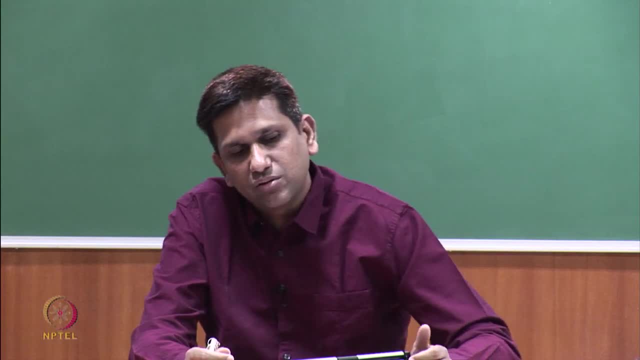 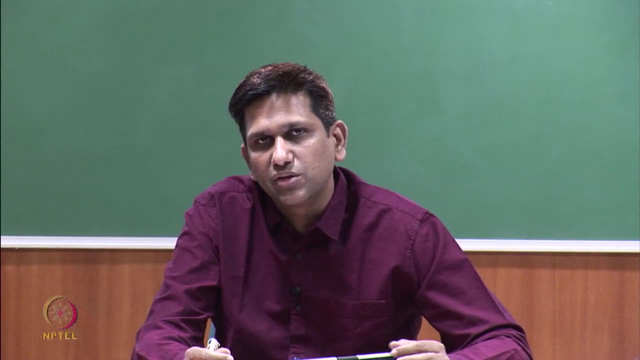 So that we have already done and later on we also solve the equation using the variation of parameter. So in that case, if I know the two linearly independent solution of the homogeneous corresponding homogeneous differential equation, then using that two solutions, that is, y1 and y2, we are 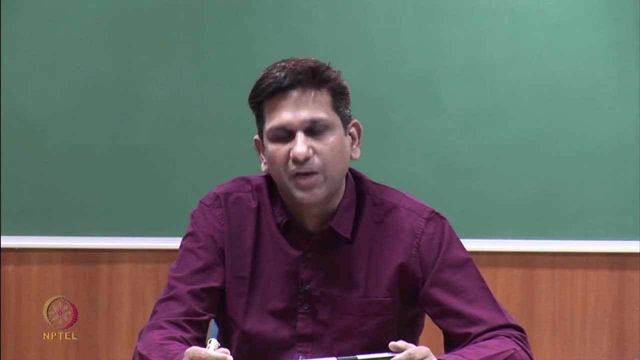 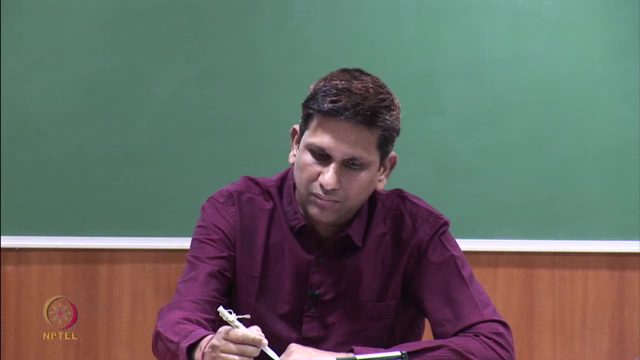 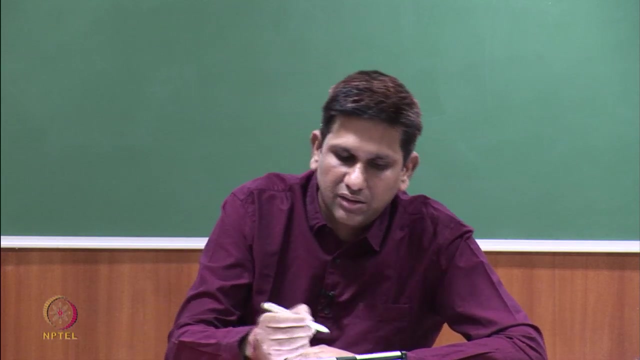 able to solve, find out the particular solution with the help of variation of parameter. So the question comes that why we are going to start with this type of problem, this type of a new method. So in this case, this method, Green's function, is useful because in we know that, if I take 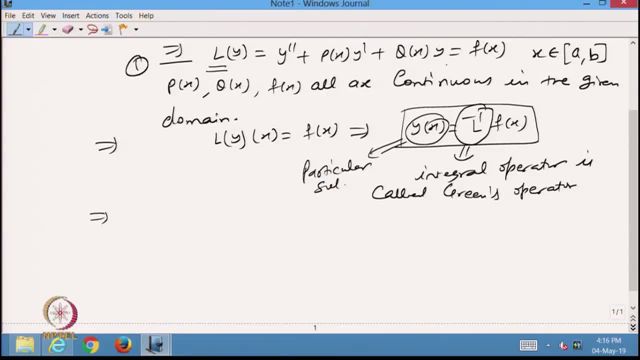 the equation number 1, my differential operator is fixed. And if I treat this equation as a initial problem or the boundary problem, so in that case also the initial condition are fixed or the boundary condition are fixed. But what about if I change the right hand side? 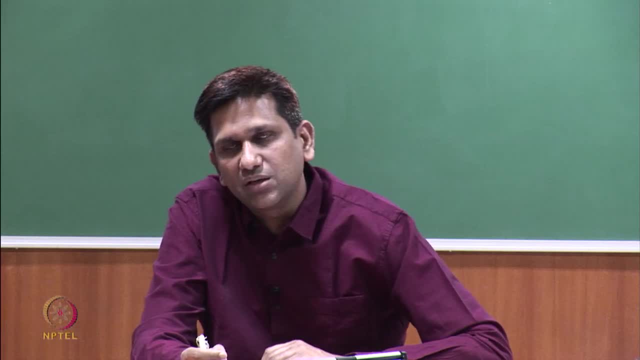 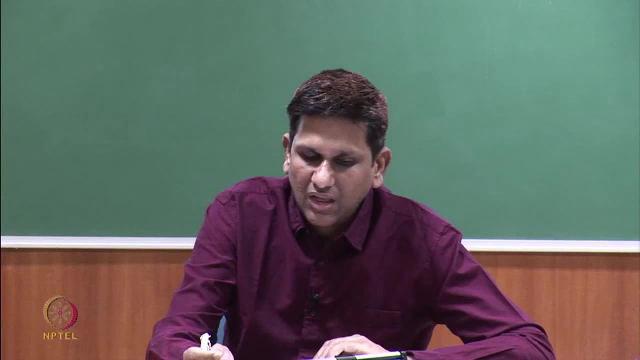 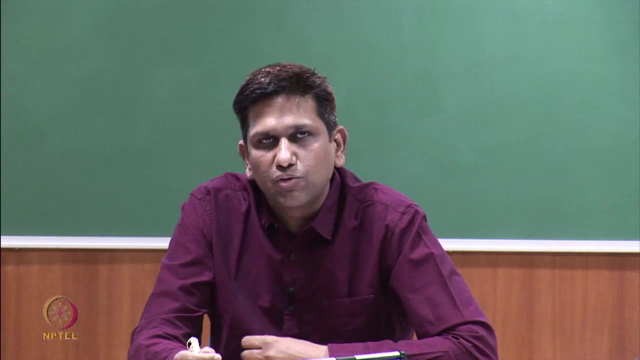 My right hand side function I change. so if I go by the previous methods, then every time the function fx is changed I have to change the strategy to find out the particular solution. So just to get rid of that one, we want to apply the method that is called the Green's. 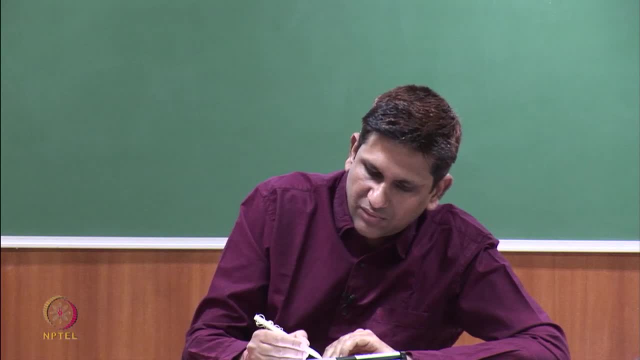 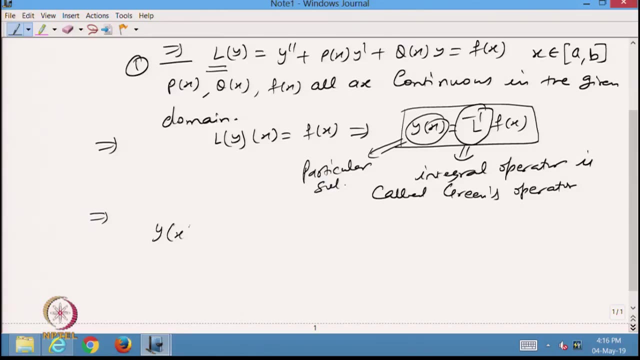 function. So now, Okay, So my solution is yx. so this operator actually we define like this one, so that is defined as g and some, so I call it g. the function of x and xi and then f of xi, d, xi and xi is: 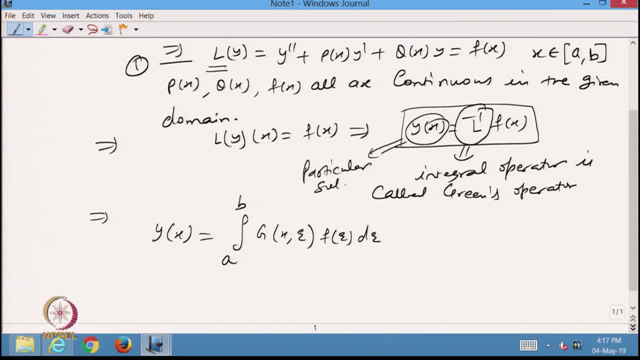 belonging from a to b. So if I do this one, This is the L inverse- and operating on the function fx. so we call it the f? xi because this is the indexing we are taking. So in this case, this is the solution of the given differential equation 1.. 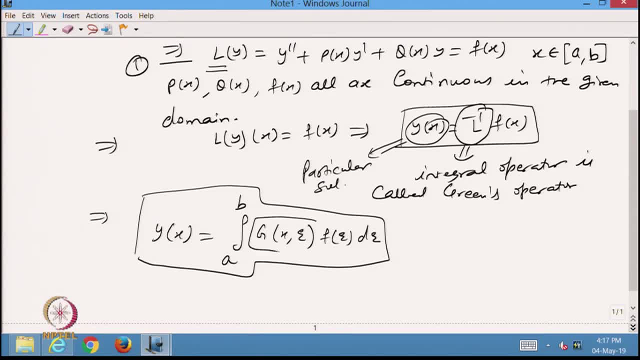 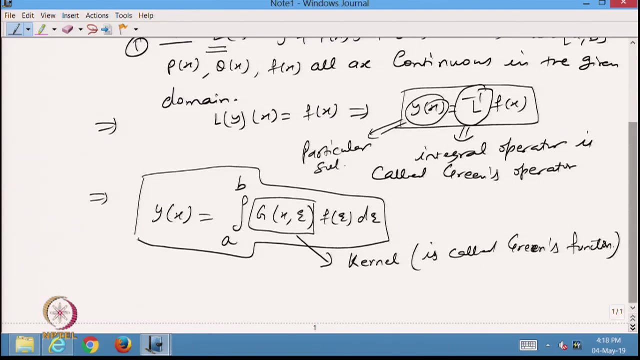 And in this case the kernel, because this is gx- is called the kernel and this kernel is called Okay, This is the Green's function. So the main thing is that, to find out, this Green functions for the given linear differential operator, So before that one. so we want to introduce a another type of function, that is, a we. 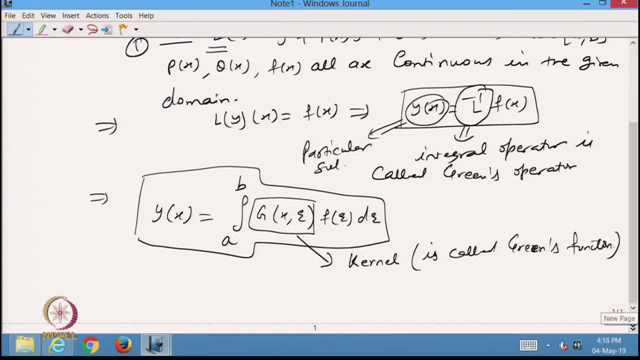 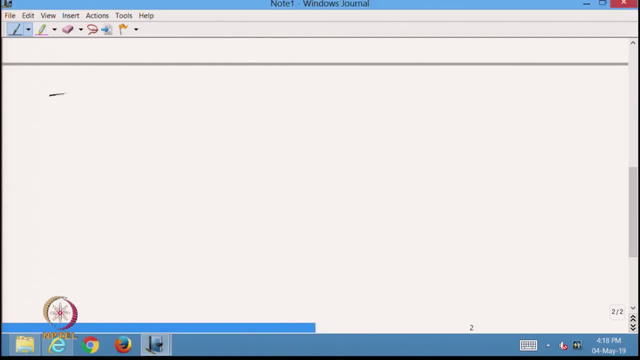 call it the special function to deal with such problem. Okay, So that is called. so I define a function that is useful for developing the theory of the Green's function and that is called step function, or this is also called heavy side step function. 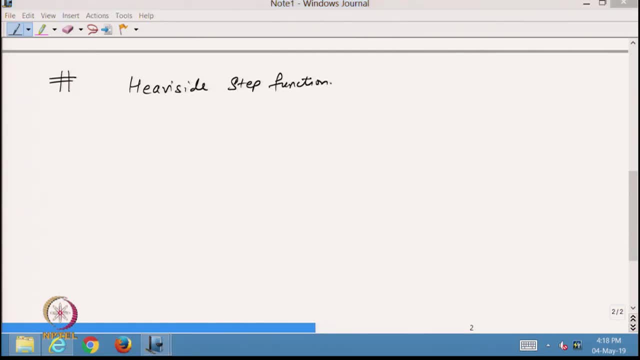 So what is that? Okay, So we define a function, we call it h, x minus a, where x is my variable and a is some fixed value. So I call it this: that this function has value 0, when x minus a will be less than. 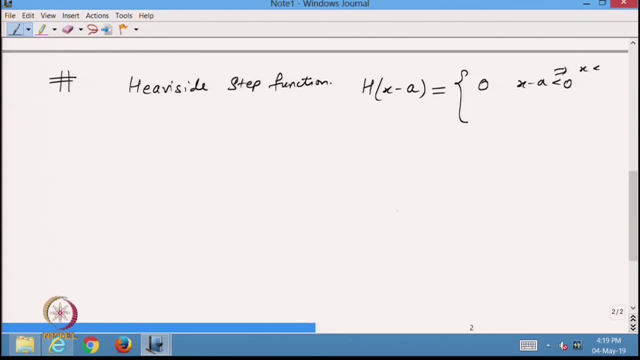 0. And from here I can say that my x is less than a and otherwise value will be 1 when x is greater than equal to a. So in this case, if I want to plot this function, so this function is look like this one: 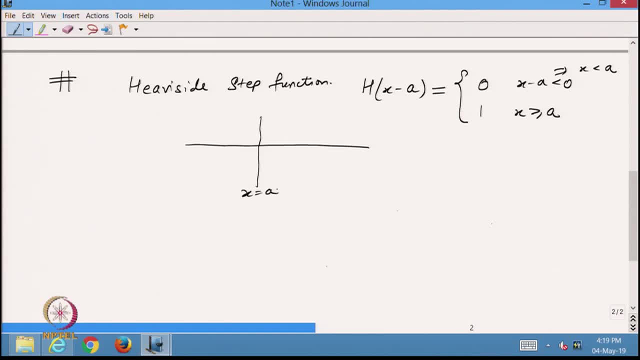 So suppose this is my a x equal to a. So if you see that this function is 0 for the whole value, So this is 0 function and at x equal to a, its value will be 1 and then its value will. 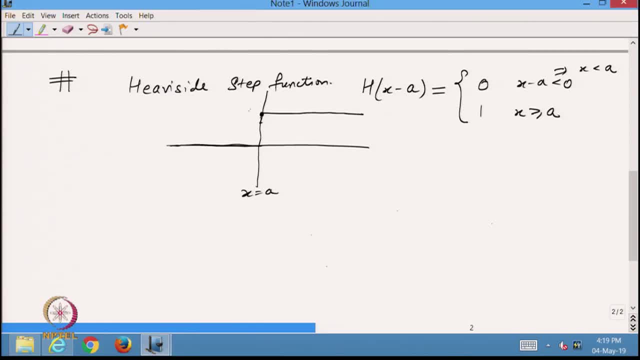 be 1 again. Okay, So this is 1, that this is a value 1, so now, in this case, if you see, then this: we have a value 0 and this value is 1, and here is a jump. 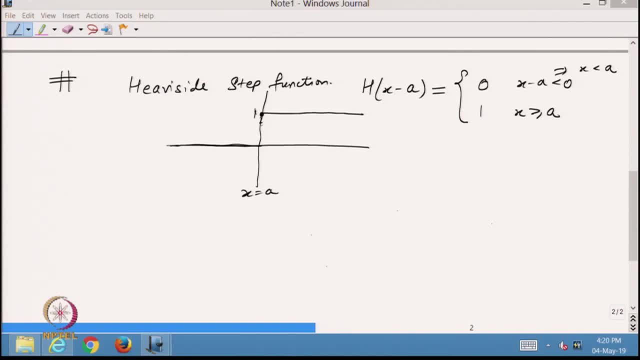 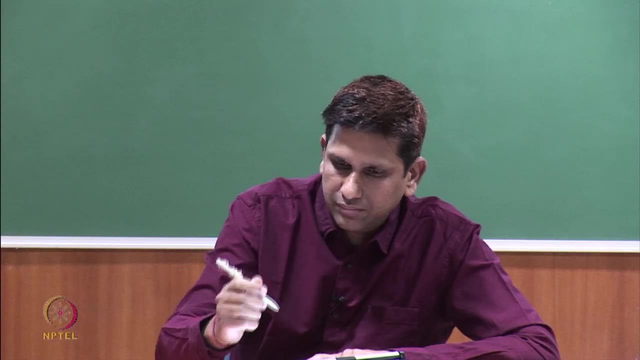 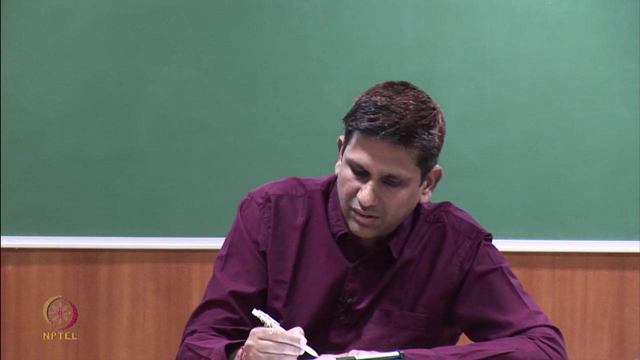 So it is also called the jump function, and we have a jump of width 1 in this case. So this is called the heavy side step function. So this function has only 2 values, either 0 or 1.. Now, so let us define another function with the help of the heavy side function. 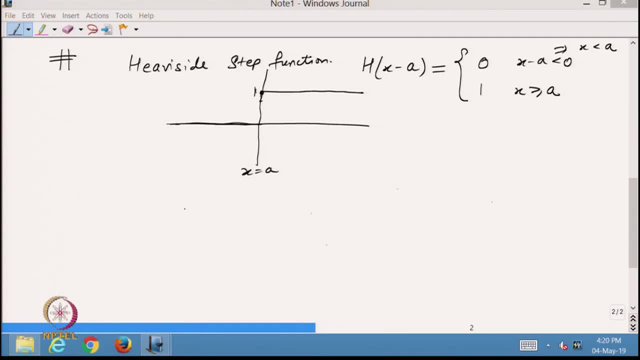 So let us see that I want to take the derivative of this function. So I just want to calculate what will be the derivative of this function, d of h, x minus a dx. So this one I want to define, Okay. 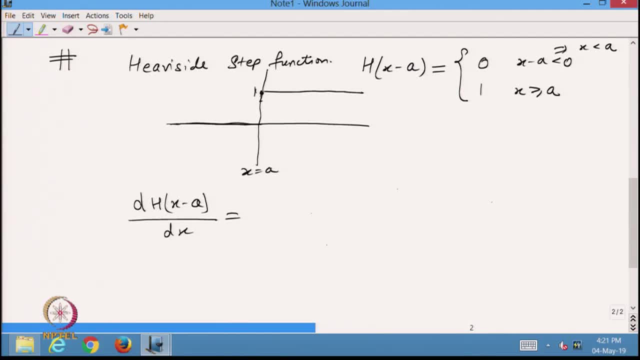 So if you see that at x equal to a, it has the jump discontinuity. So, but if we take the x less than a, this is the function parallel to x axis, so its derivative will be 0,. after this, x equal to a greater than a, its value will be always. 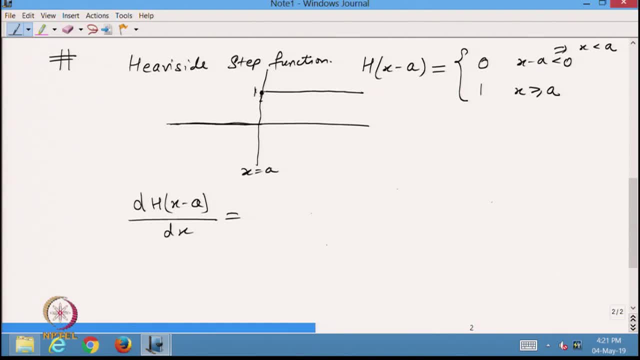 the derivative will be 0, because this is a parallel to x axis and here we have a jump. So here, if I want to find out the slope of this one, so that is infinity. So in this case, this will be 0. 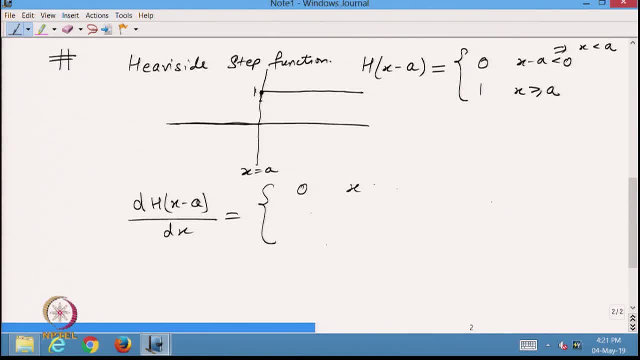 Okay, So this will be 0 when x is less than a, this will be infinity when x is equal to a, and this will be again 0 when x is greater than a. So with the help of this function, this value, we define a function, and then that is called. 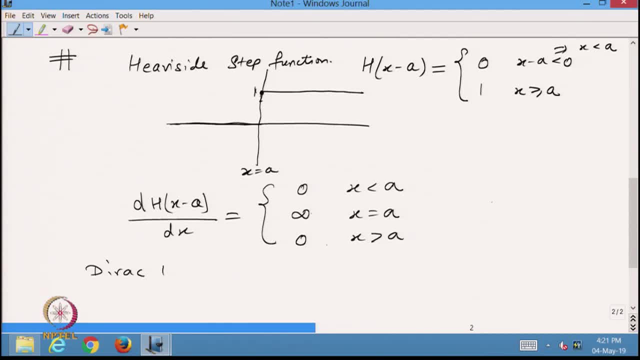 Dirac delta function. This is called Dirac delta function. Okay, Okay, So this is by the physicist, that is the Dirac. So in this case we define a Dirac delta function. So I define a Dirac delta function. delta x minus a. this is equal to, if I call it. 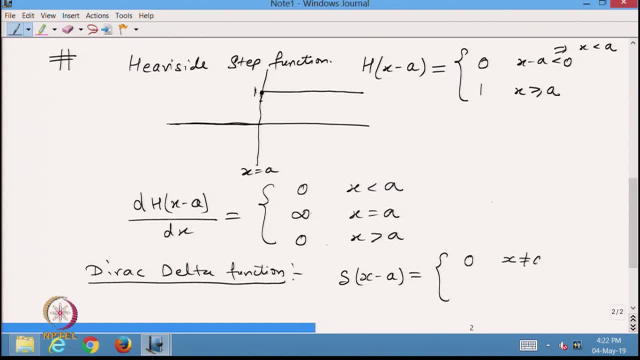 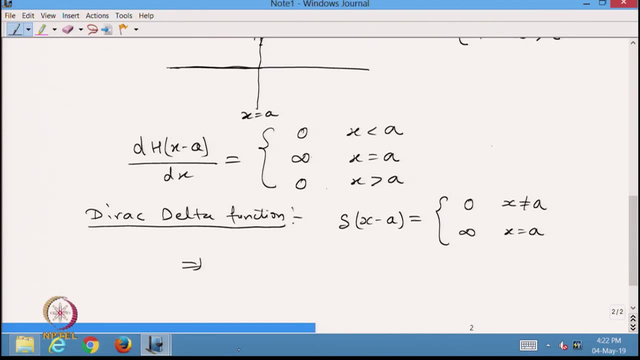 that a 0, when x is not equal to a. because if you say here x is less than a or x is greater than a, its value is 0,, otherwise its value is infinity when x is equal to a. So from here I can say that Dirac delta also can be written as the derivative of d. 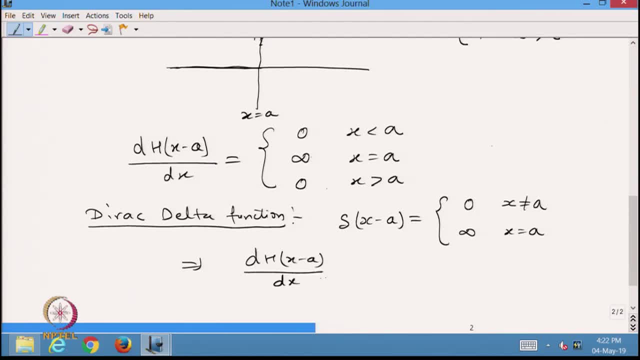 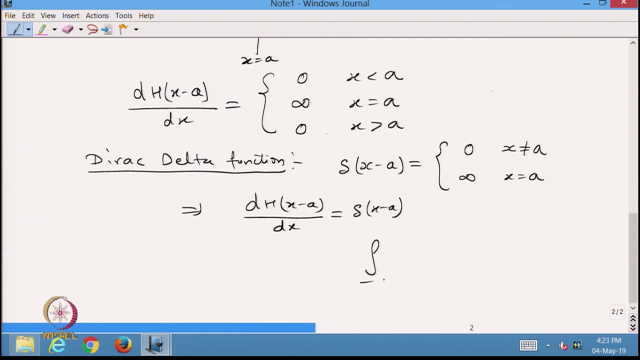 the Heaviside function dx, and that can be written as a Dirac delta function. So this is the function. Okay, And the this function has the property that for the Dirac delta, that if I take the integral from minus infinity to infinity of this function, x minus a dx, then its integral is equal to: 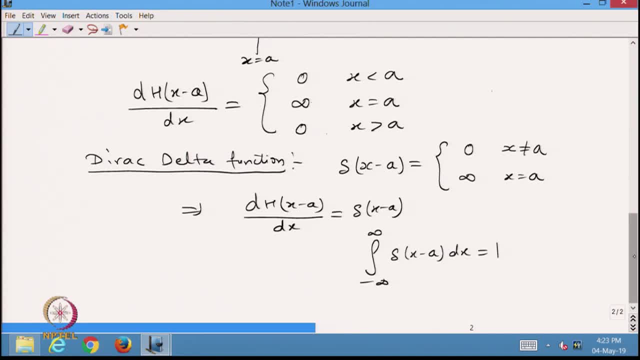 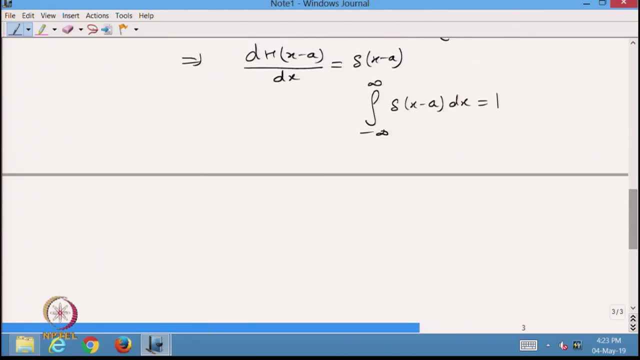 1. So if you just want to define this function, because this function, if you want to draw, then you will see that. suppose I take this function, Okay, This is my function, and let a is equal to 0, so in this case, this a is equal to 0 and 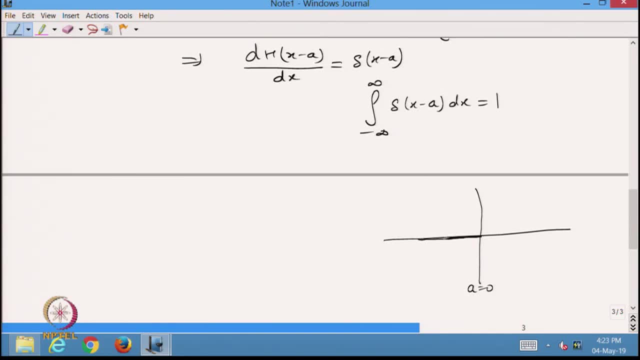 so the function is 0 everywhere. this is 0, only at this point its value is unbounded. it is going very high, so it is unbounded. So this function has a 0 value. everywhere Except a, I have taken a equal to 0. 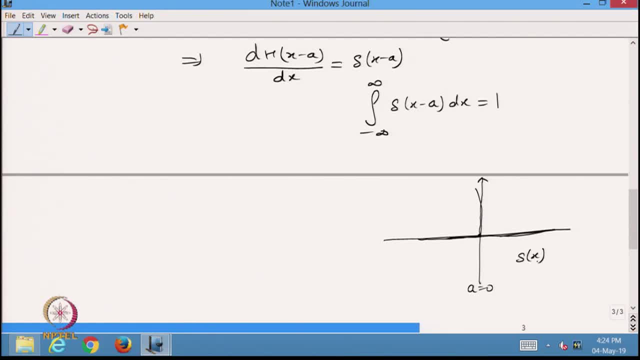 So in this case, my Dirac delta function will be delta x. So this is the function. we can draw little bit about the Dirac delta function. Now the thing is that we want to prove this property. So for this one, because this is a special type of function, I define this function as: 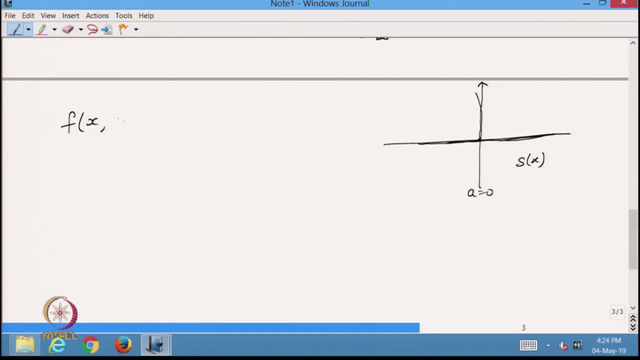 a new function, f, That is x. Okay, So this is x and I define a new parameter, epsilon, so I define this function as a another function. So this function I take as so this is I take a width interval, of width, so minus. 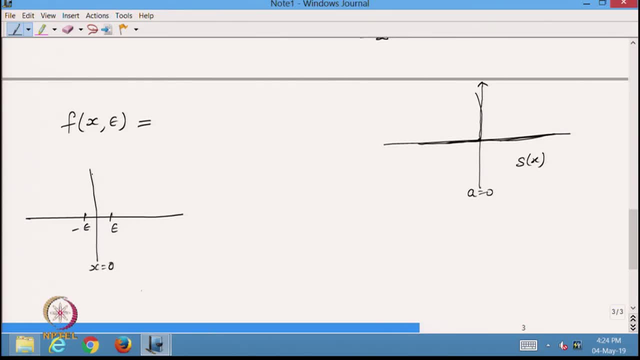 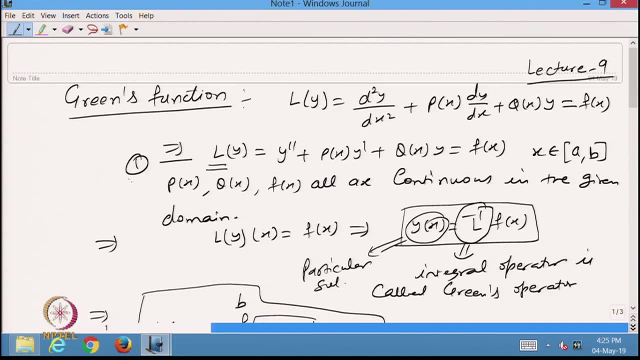 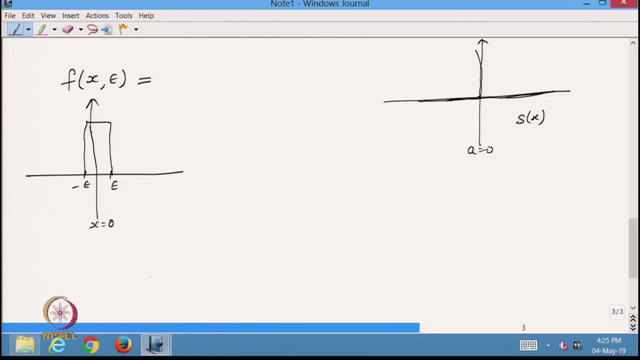 and this is x equal to 0.. So, in that I define a function, So this is a function whose width is so this function I am defining, so this function, So my f, x, in this case I take the width, that is 1, over. so I define this function. 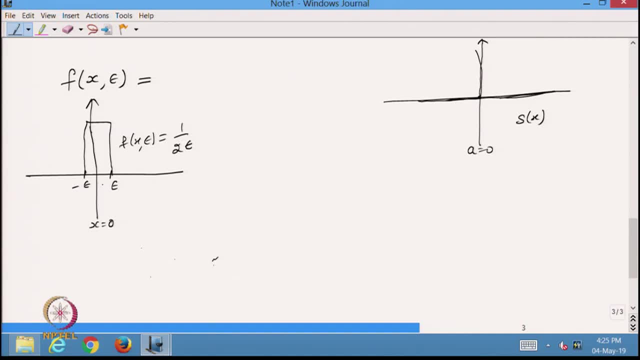 like this. Now it is just the. if I start taking the epsilon tends to 0, then this function tends to infinity. So in this case, this is the width of the function and that is the height of the function. So I define this function as this one. 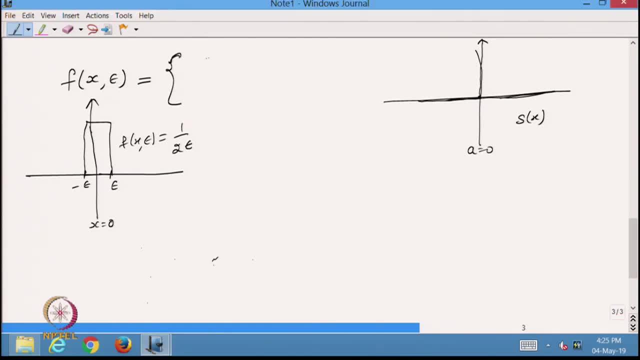 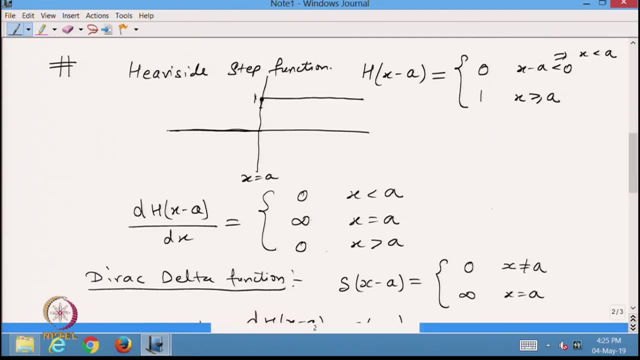 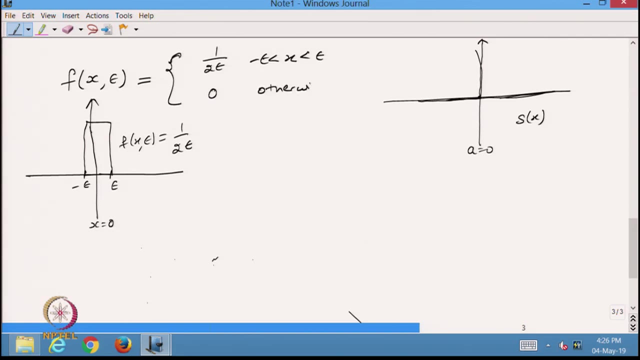 So I define the function: f, x is equal to 1 over when my x belongs to minus pi to pi, and otherwise its value will be 0 when otherwise. So this is the function. Now, if I take this function and I want to integrate this function from minus f, x, epsilon, 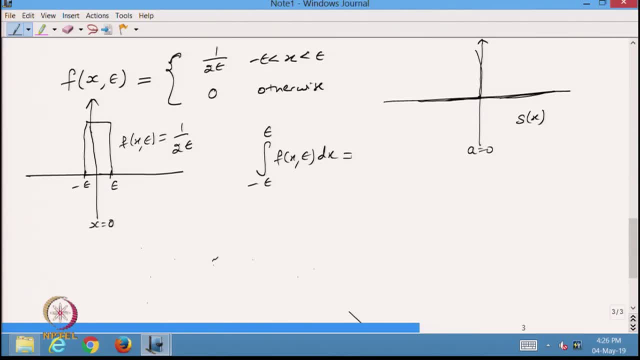 dx, then if you see this one, that the integral, I want to define this function. so this function is a positive function. So basically, I want to find the area of this function under this curve. so from here I can say that. 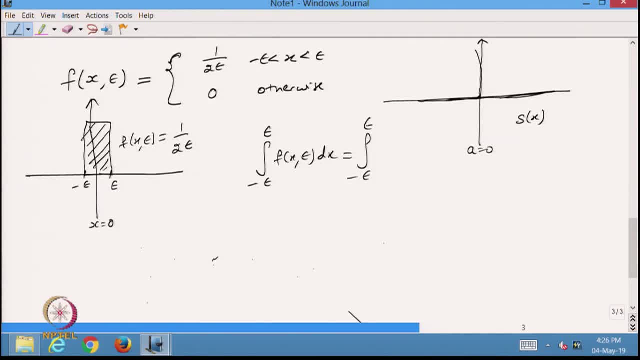 x is around x Maya, 1 over 2 epsilon, dx, otherwise value 0. So this will be again 2, 1 over 2 epsilon. and then this will be x, So it will be 2 epsilon into 2 epsilon, So its value will be 1. Because 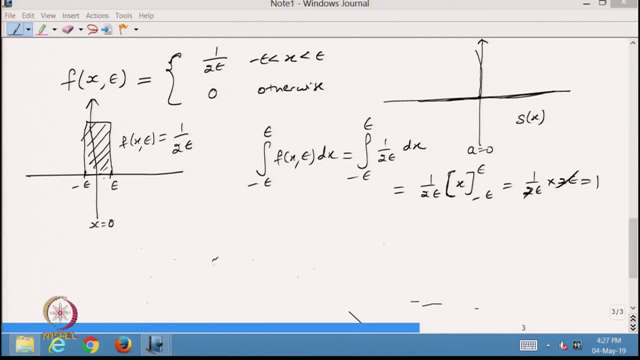 in this case I have the width of width of that the length, 2 epsilon and the function is 1 over 2 epsilon. So if I multiply that value becomes a 1. The same thing I can apply for this function. Suppose I apply this one for minus infinity. 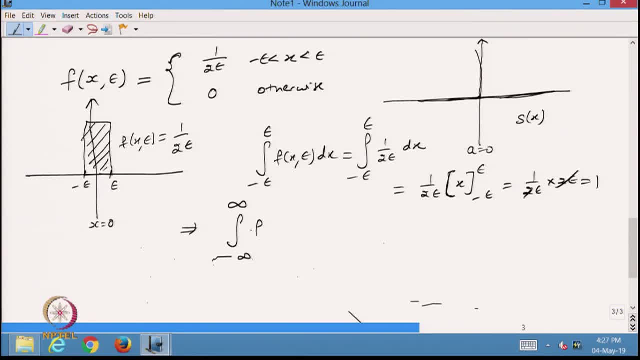 to infinity, from minus infinity to infinity, dx. So this one I want to define. So if you see this function, I can write in this form: from minus infinity to minus epsilon, F, x, epsilon, dx, plus, minus epsilon to plus epsilon, and then from epsilon to infinity. 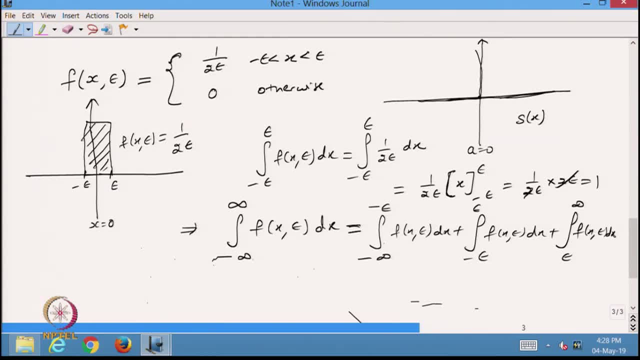 F, x, epsilon, dx. So in this case, this is the value of this function. function is 0 from minus infinity to epsilon. this value 0, this value 0 here. So from here I can say that this will be 0 plus minus epsilon. 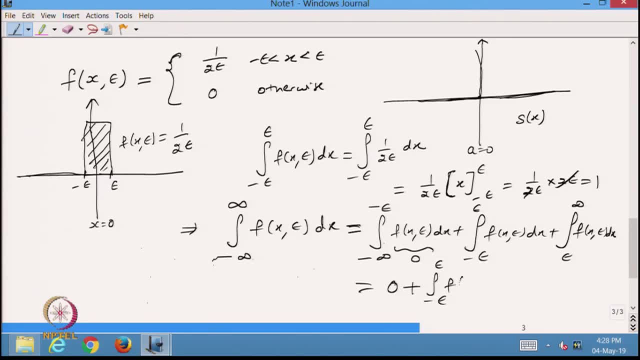 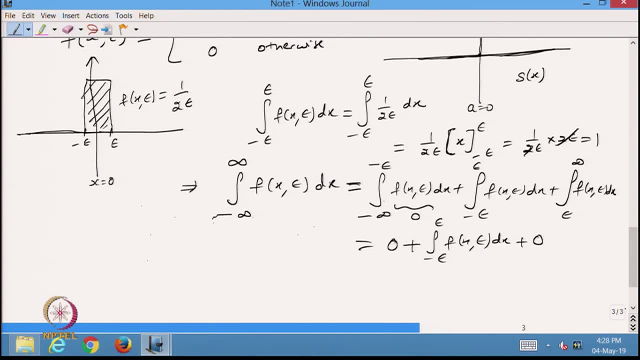 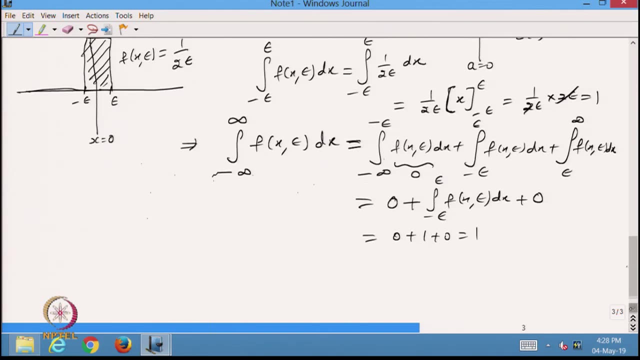 from minus epsilon to epsilon: f, x, epsilon dx plus 0 and this value. we already know that this integral is 0 plus 1 plus 0, so this will be 1.. It means that if I integrate this function for the interval minus infinity to infinity, its value is also equal to 1.. Similarly, 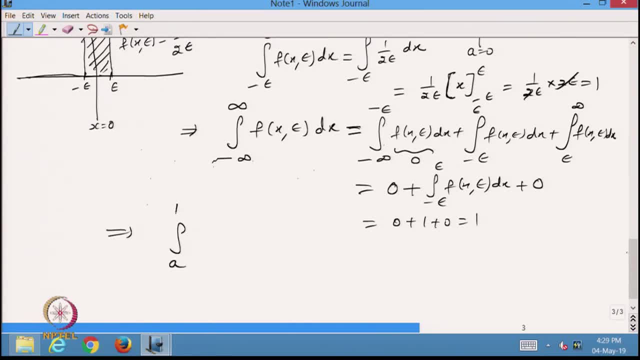 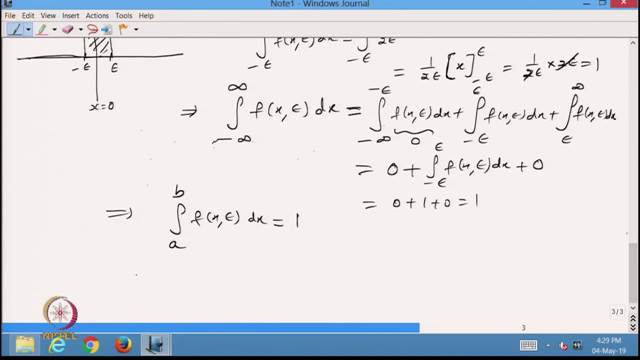 I can do for a finite interval from a to b. Yes, Yes sir, Yes, Yes sir. So in this case, value, the same way I can define, and its value will be again 1.. Now, if you see, from the function I have defined, if I take the limit, epsilon tends to 0, f of 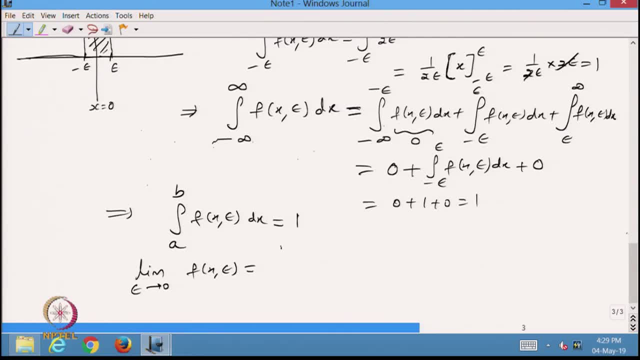 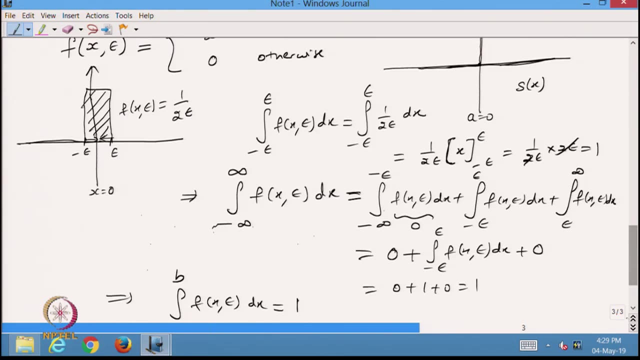 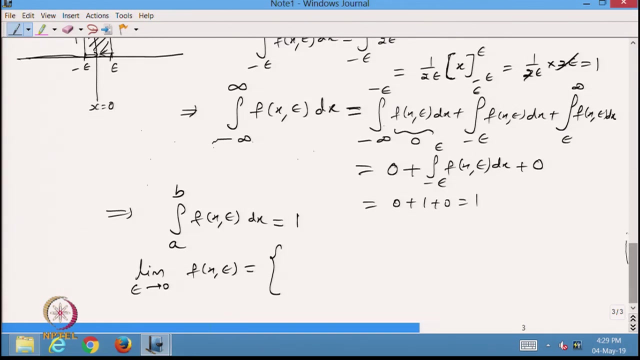 x epsilon. So if I apply this limit, then you can see that this width is going to decrease and becoming 0, then the height of the function, the height of the function, is going to increase and it going to become the infinity. So if I put the limit, epsilon tends to 0. this one. 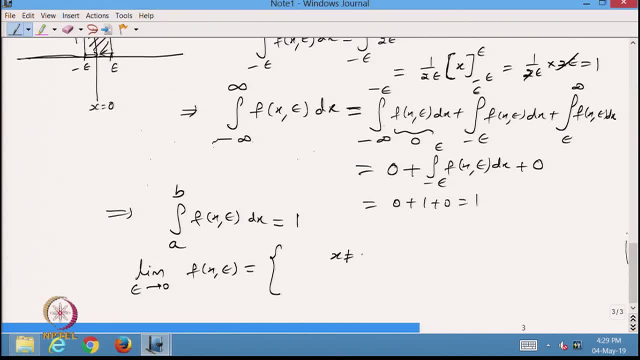 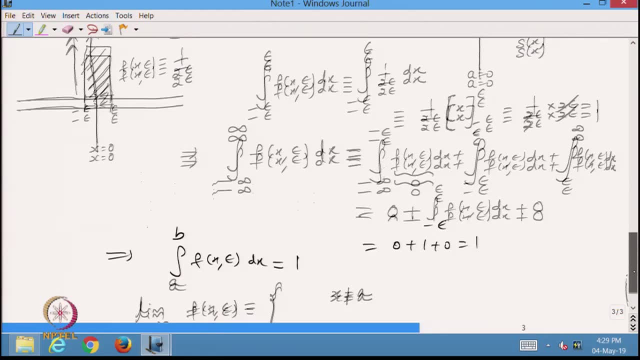 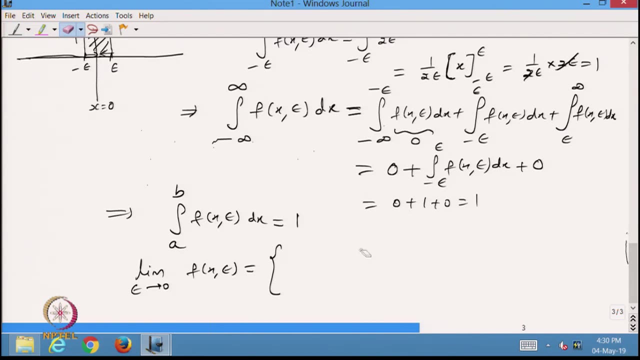 then I can say that when x is not equal to a, So in this case I have defined the function f of x, this value, So this value will be 0 when x is not equal to 0 and become infinity when x is equal to 0, because this function, if you see this, is a function. So when the epsilon 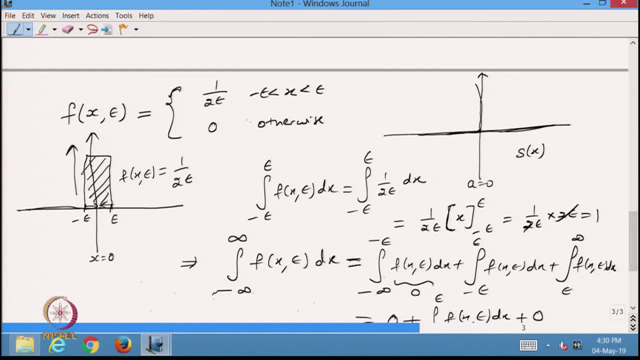 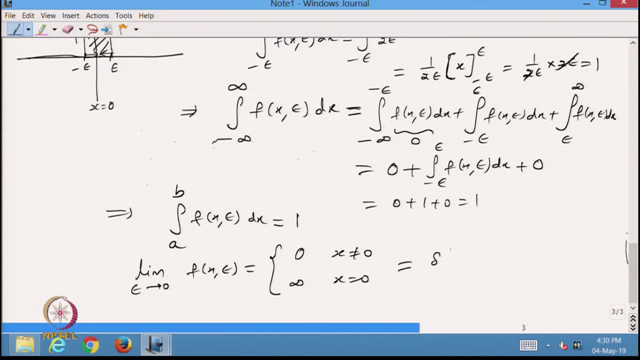 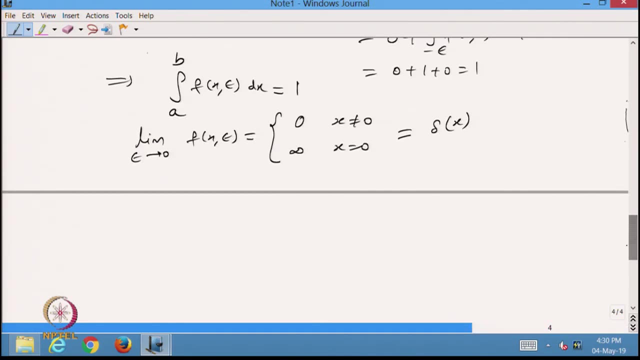 turns to 0, we are heading toward the x equal to 0, its value will be infinity, other words, value 0.. So basically, from here I can say that that this is equal to a Dirac delta function. So from here I can say that. so from here, one thing is there that the limit epsilon. 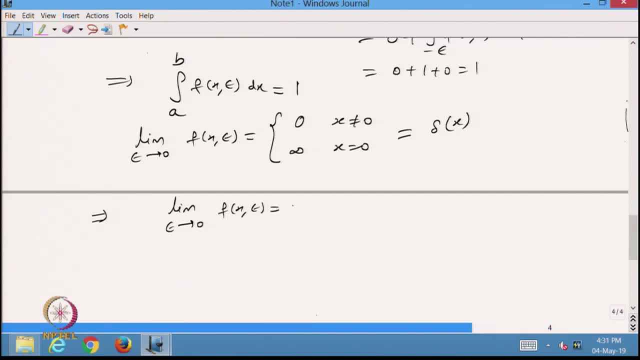 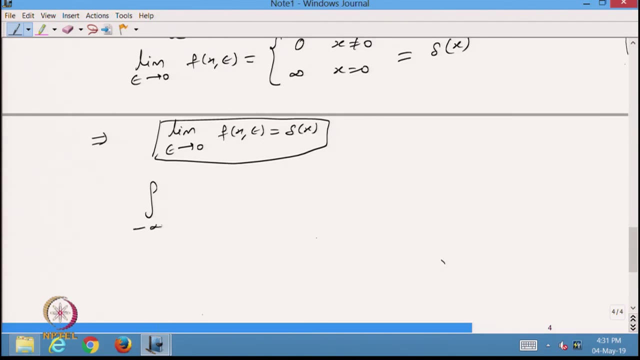 tends to 0. f of x, epsilon is equal to Dirac delta. So this is the definition of the Dirac delta. Now I want to define that. what about? I know that, from minus infinity to infinity, my function Fx, epsilon dx, its value is equal to 1.. So 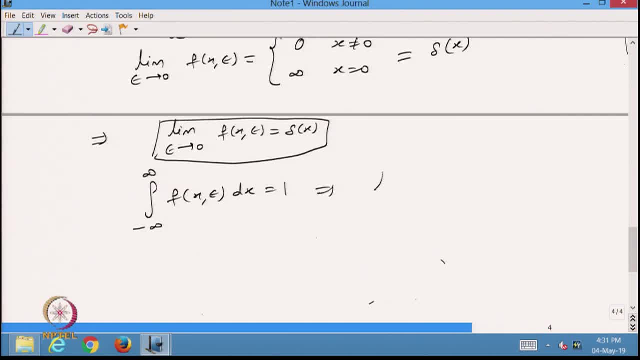 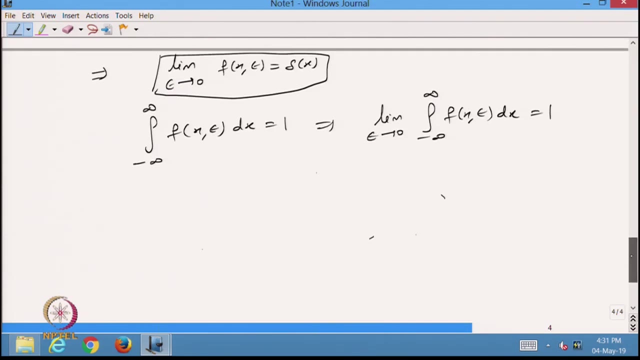 just now. we have done that one. So now what we do? I take the limit. So limit epsilon tends to 0, from minus infinity to infinity. f of x, epsilon, dx, and this is equal to 1.. So by the Leibniz test I can take this interval. 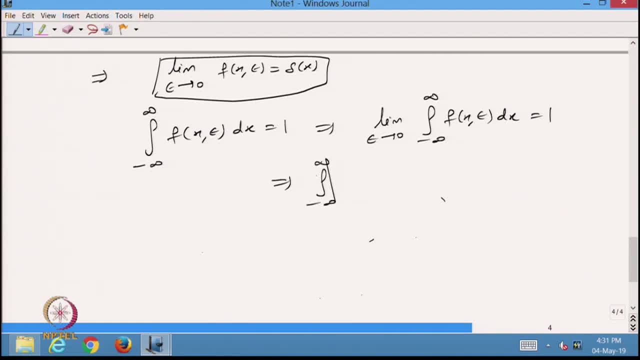 this limit inside, and this will be so, this one will be minus infinity to infinity. then the limit f of x, epsilon, dx, and that is 1, and I, just now I have defined that this is equal to the delta function. So from here I can say that is minus infinity to infinity. 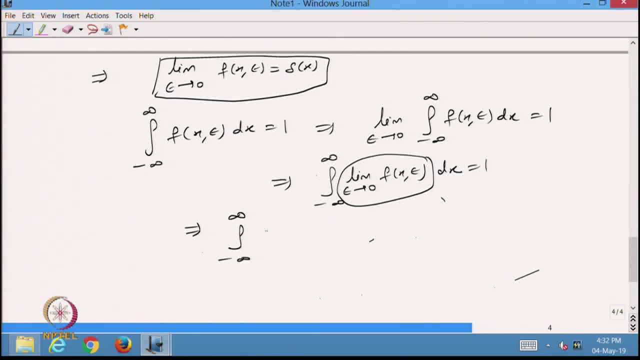 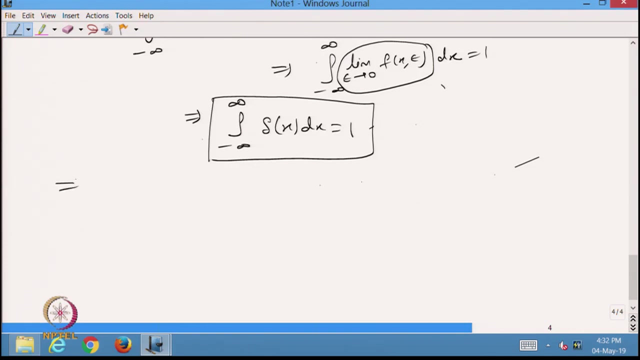 it is the delta function: x, dx- that is equal to 1.. So this is what we want to want to prove. So in this case I have taken the value: a is equal to 0 and the same way I can define for the shift function. 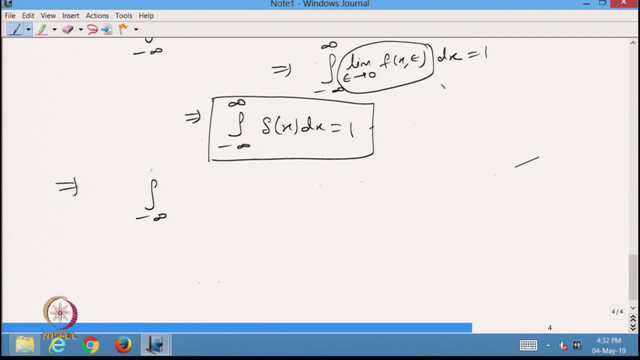 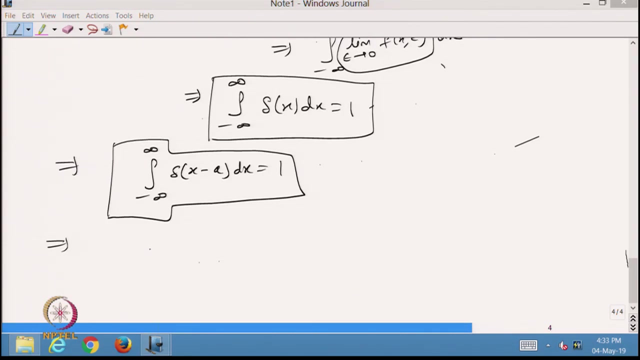 So the same way I can define that minus infinity to infinity delta function, minus a dx, that is also equal to 1.. So with the help of this one, so this is we are able to prove. Now the next thing I want to prove that is will be useful in future- that what about this one? if I take 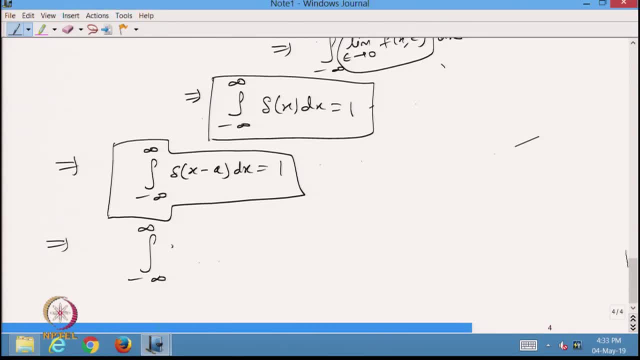 the interval from minus infinity to infinity: x minus a, and then I define f, x, a, dx. So this will be what In this case, what we are doing, that we are taking the drag delta function and multiply by function f, x, and I want to see that what will be the value? 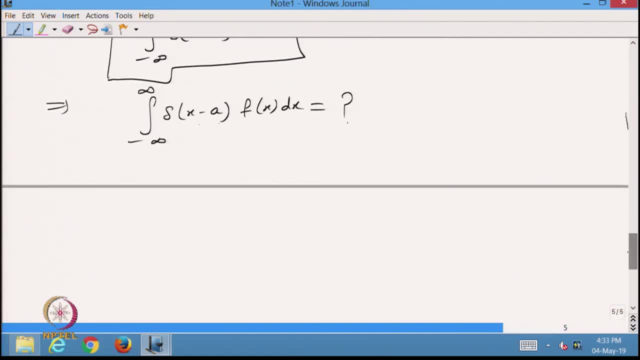 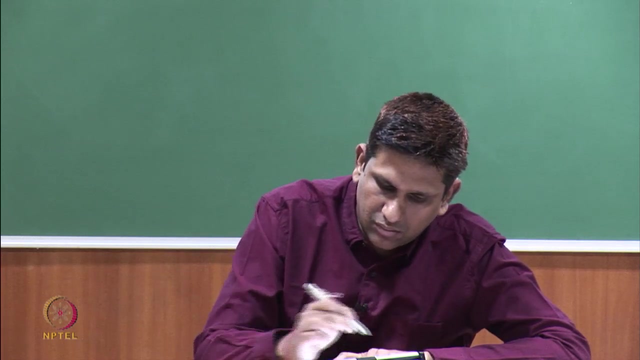 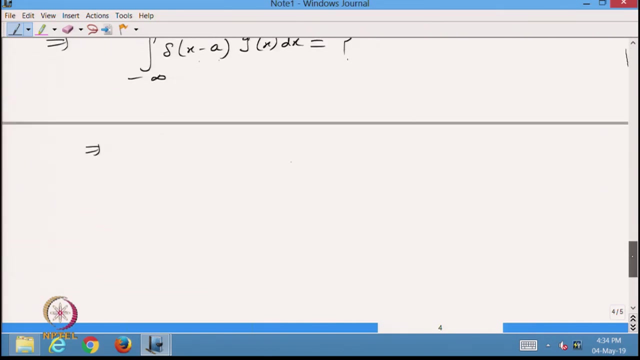 of this one. So this one we will prove now. before that, I just want to prove that, taking the same function again that we have defined. So in the last one I have defined, just take, I just want to write this as a g function. 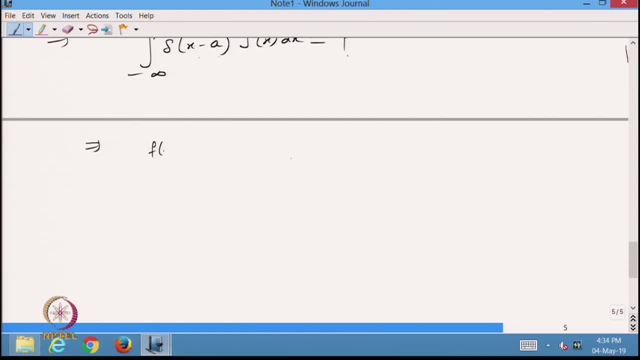 Now I want to define that. what will be the function f x epsilon into g x? So this will be: if you see, this will be g x by 1 over 2, simple by square root of 1, 2,, 2, 2 plus. f x epsilon into g x. So this will be, if you see, this will be g x by 1 over 2, 2, 3, 2, 2, 4, this will be the value of the function f x epsilon into g x. So this will be, if you: 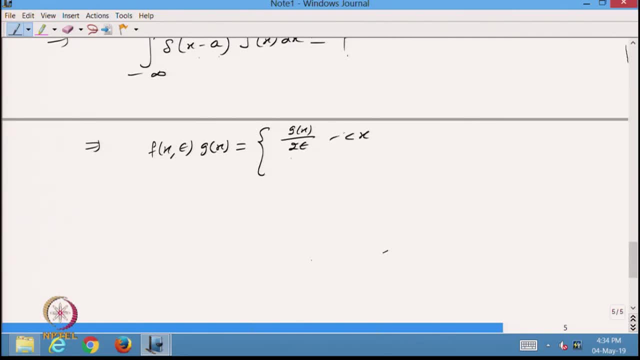 see this will be g x by 1 over 2, 2,, 3, 4, this will be As in you have take this is California over 2 epsilon, when x is from minus epsilon to epsilon, and this will be 0, otherwise, right. 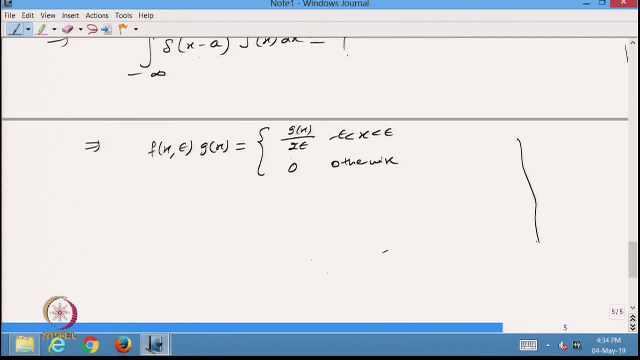 So in this case, so this is my function and so this is my x axis and this is the axis I am taking y axis. Now we have defined a function, So this is minus epsilon and this is plus epsilon. So in this case, now I have defined another function, So this function. 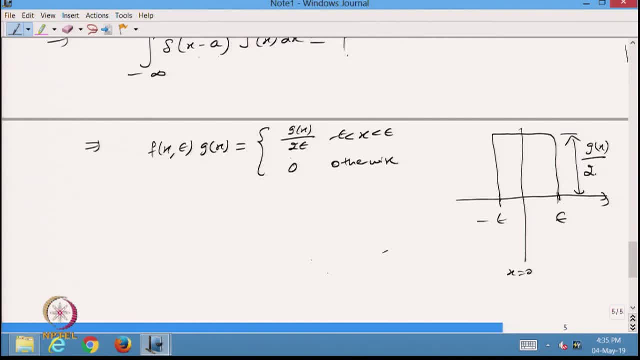 is g, x over divided by 2 epsilon. So this can be another function. So in this case I just want to define that. what is the x And area under this curve? So I want to find out what will be the value if I take the integral. 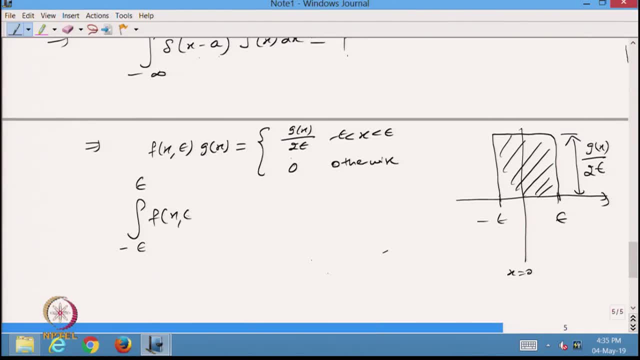 from minus epsilon to epsilon f of x epsilon dx, g x into dx. So we know that this will be. So this function we have defined. So this value will be g x over 2 epsilon dx. Now the g x is a function, So this function can. 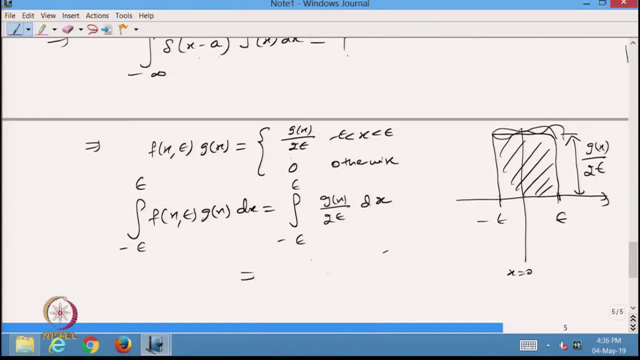 be of this type. this can be of this type, but this is a continuous function in the given domain, So it is integral function. So what do we do? that? I approximate this function, the height of this function, but the value at this point, So I can approximate this. 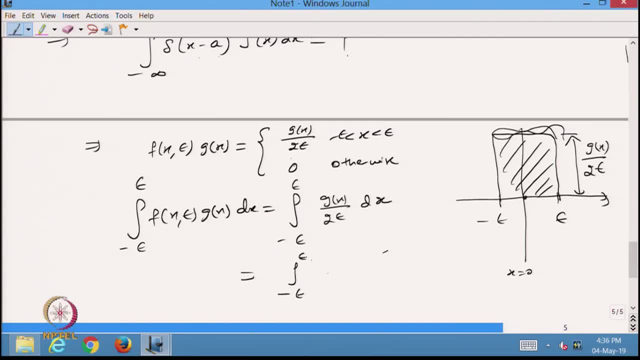 function as minus epsilon to plus epsilon and I approximate this function as g at x equal to 0, because I have defined the function. I am taking the interval about x equal to 0. So I just take the value, the function, as approximate value at g at x equal to 0 divided. 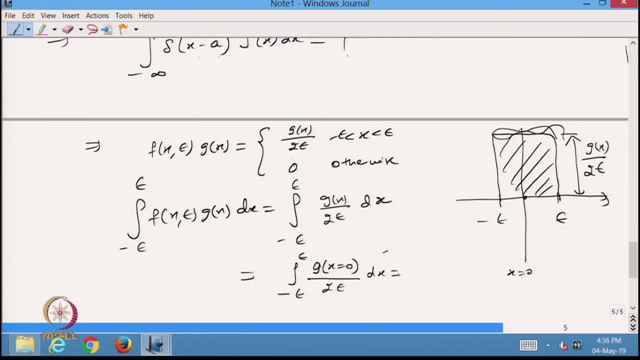 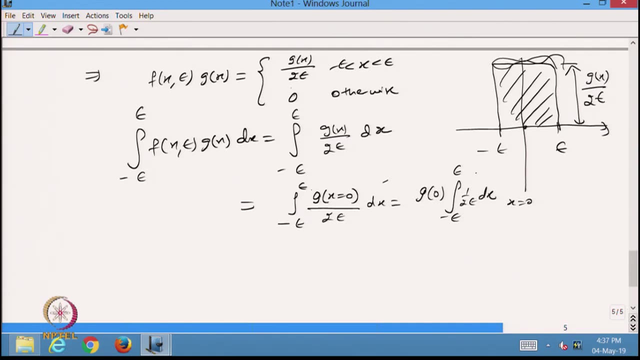 by 2 epsilon dx. So from here I will get the value, and this is minus epsilon to epsilon 1 over 2 epsilon dx, and from here this value. I already know that this is equal to 1.. So from here I can say that this will be equal to g of 0.. 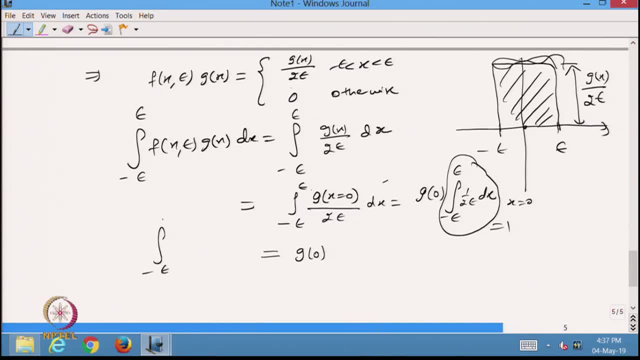 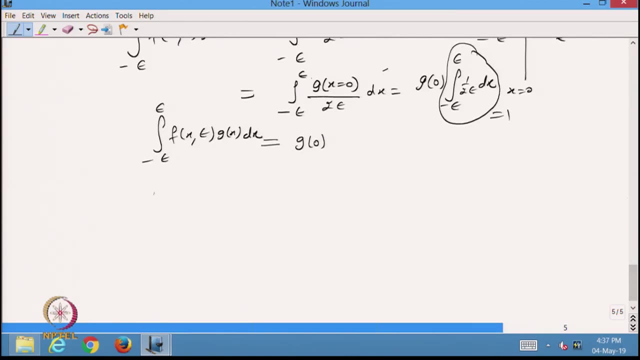 Okay, So f of x, epsilon, g, x, dx. So this will be the value of the function here. Similarly, I can define this one for minus infinity to infinity: f, x, epsilon, g, x, dx. So in this case also I can define this value as g. Now I just define the value of the direct delta function. 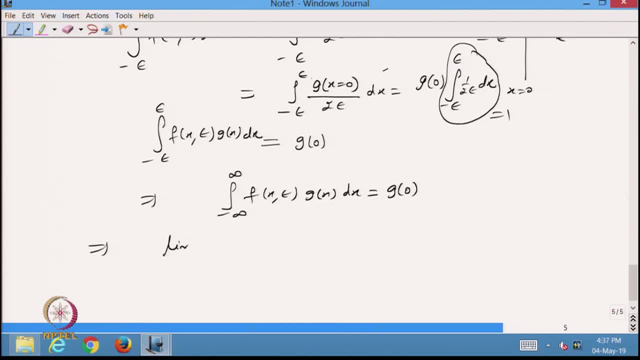 So I also know that if I put the limit, epsilon tends to 0 for this integral g x dx. So this will be again. So that becomes the direct delta function. Okay, Right, And it will be equal to x. that is, x into g x dx and this value is: again it will be equal. 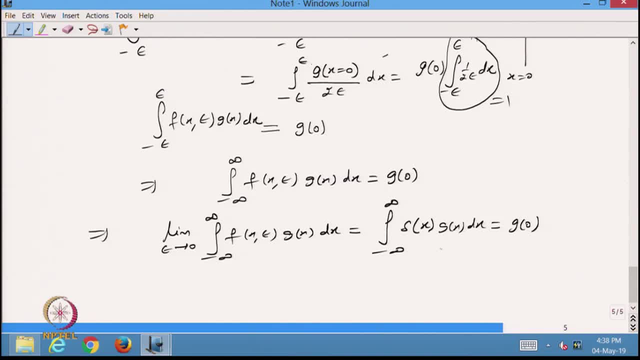 to g 0, because I have defined the Я can be a mean just minus f, the function at 0.. So from here I can say that if I take the integral from minus infinity to infinity, drag delta x minus a into g x, dx, So in this case this value will be equal. 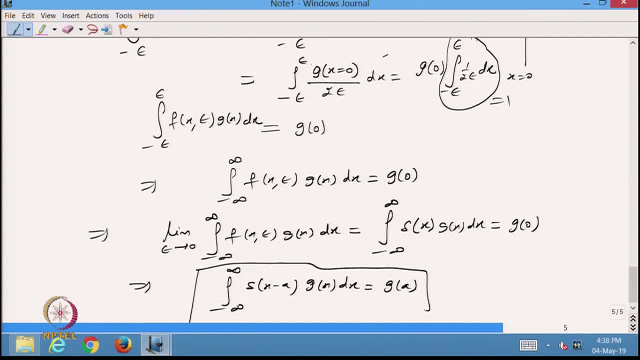 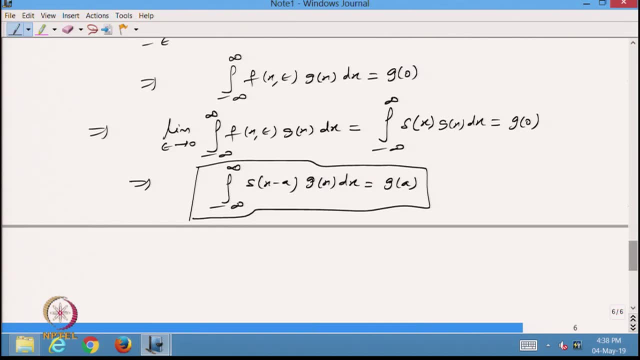 g, Absolutely, is very one of the important integral or the properties of the Green function. So that is, we are going to use a lot for defining the Green's function. Similarly the same property. I can define that from a to b over this finite interval. 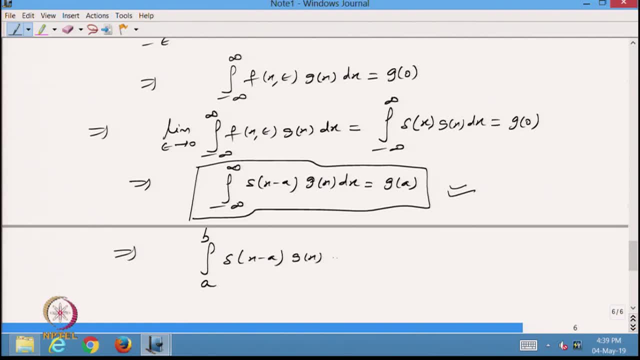 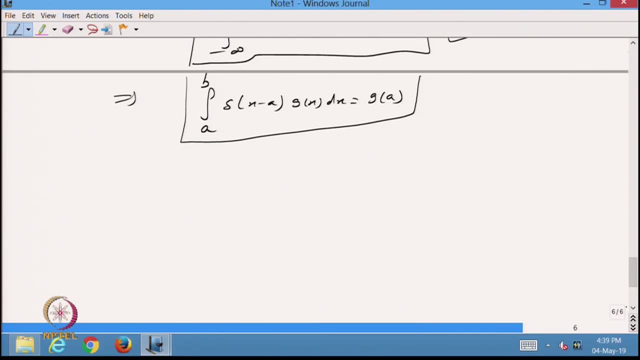 the drag, delta and gx, dx, So that can be written as, again, the ga. So this is for the finite domain. So now, after doing this one- so let us start that- how we can define the Green function for the given linear differential operator. 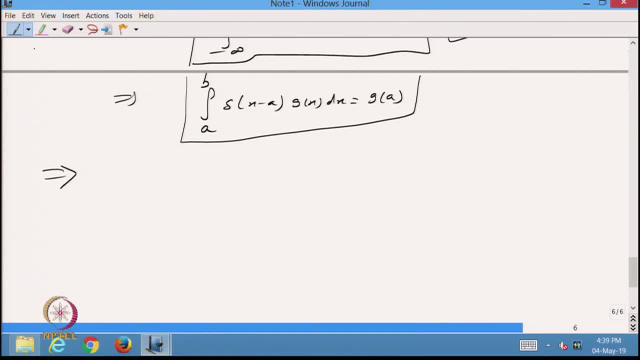 So that I the L, the differential better I know. so that is operating on the function yx. this yx is the function, is a, continuous. basically this belongs to c, to a, b and that is giving me equal to fx. Now I want to define that. let L of I define the function g. So let us define l of g. So I want to define g of g. So that is: I want to define g of g. So that is. I want to define g of g. So that is. I want to define g of g, So that. 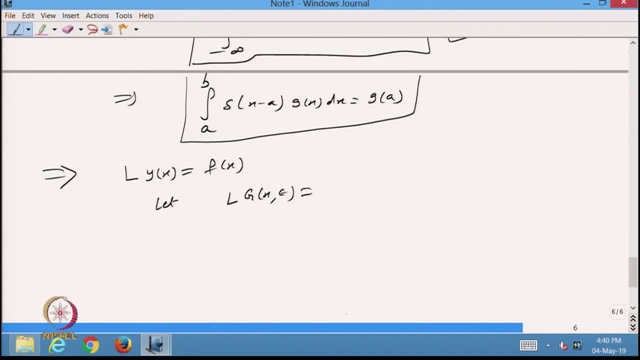 g, that is, the green function, is equal to drag tilt. So this is the function I am defining and this function is defining. So let us define this operator that, operating on the green function, some g, x, epsilon or epsilon. instead of epsilon I can put the xi, because 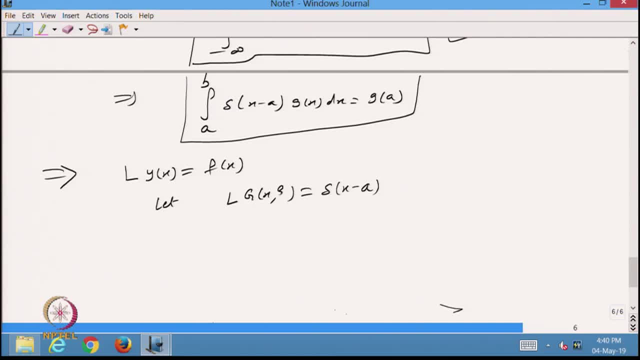 we are dealing with the xi here and that is equal to. I put x drag delta function: x minus xi. So now I know that this function can be written as it would be 0 when x is not equal to xi, and this will be infinity when x equal to xi. 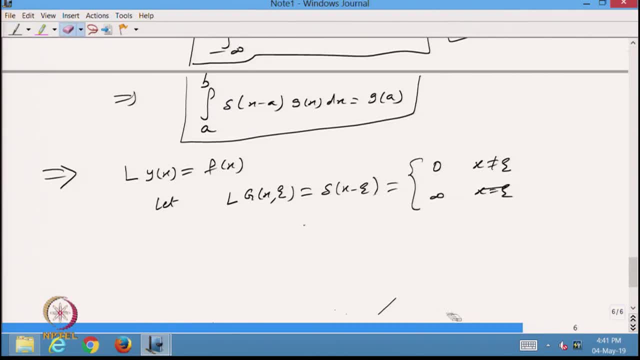 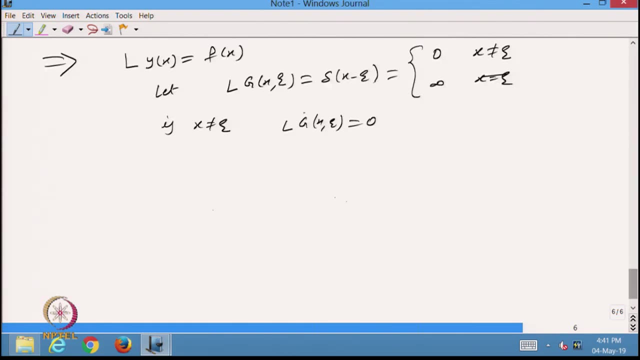 So in this case, we know that if x is not equal to xi, then so if x is not equal to xi, then my v equal to 0.. Now, if I have this one, and we have defined that with the help of the green function, I can define my. 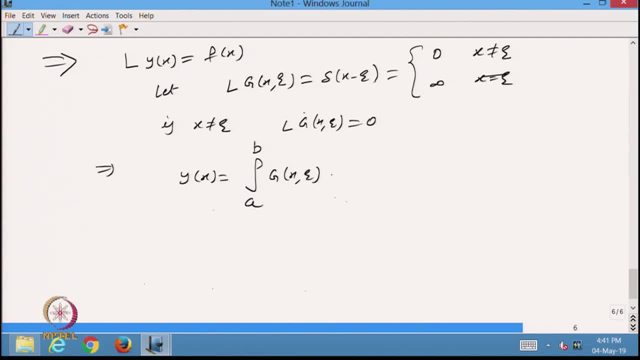 In, So this will be f, x. So this will be f of xi, d, xi. So that is the solution we have defined. So let us see what will happen here. I operate this one with the L, So L of y. 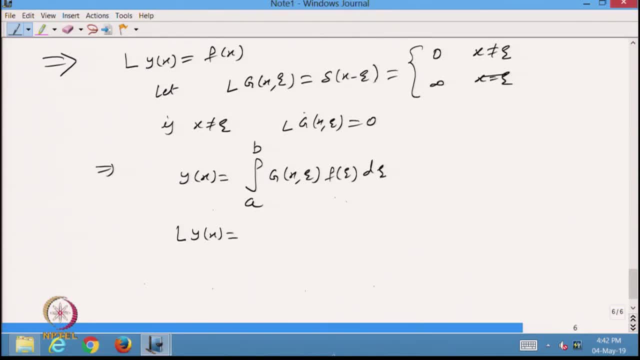 x will be L, defining on this, operating on this integral. So I can take this operator inside with the help of Levene's theorem, So from here I can write. So this will be L of g, x, xi, f, xi, d, xi. 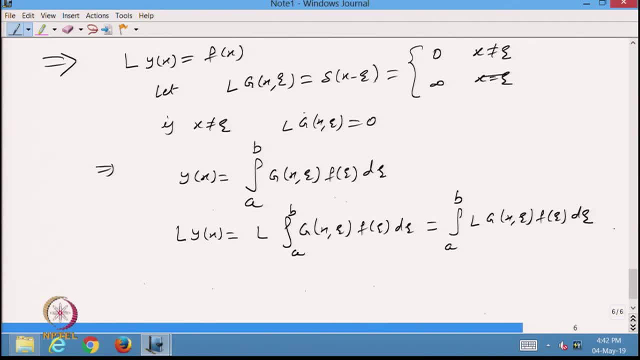 Because a and b are the constants, so other term will be 0. And this will be again a to b and LG we have just defined that is equal to the drag delta function. So this will be x minus xi, f, xi, d, xi And this one we have defined in the previous slide. then that 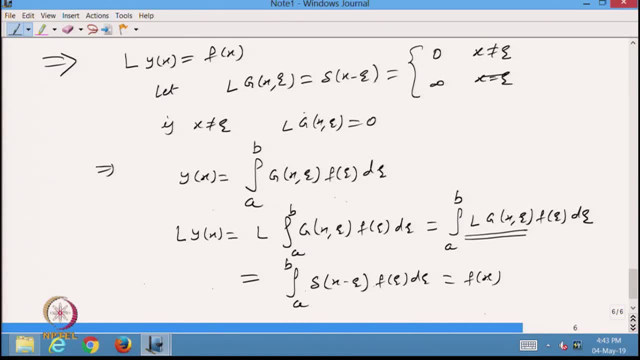 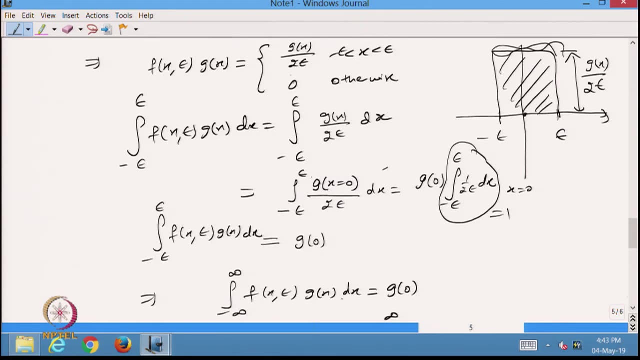 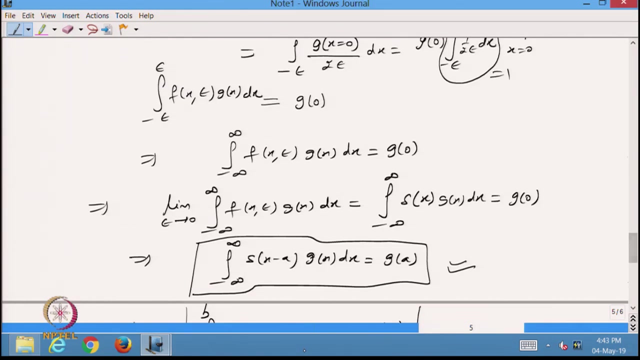 this will be equal to f of x, because I am applying the delta x minus xi and we are taking the integral with respect to xi. In the previous one we are taking the here, so we are taking the integration with respect to x like this one. So here we are taking the integration with respect. 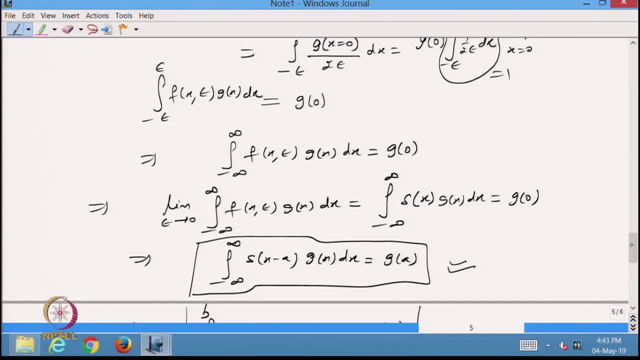 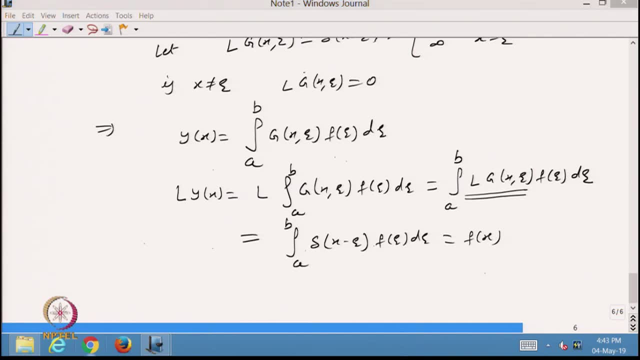 to x and we will get the value ga here. So the same thing is coming here. So in this case I am taking the integration with respect to xi, so I will get the fx. And what is this? So from here I will get that my l of yx is equal to fx And that is the given differential. 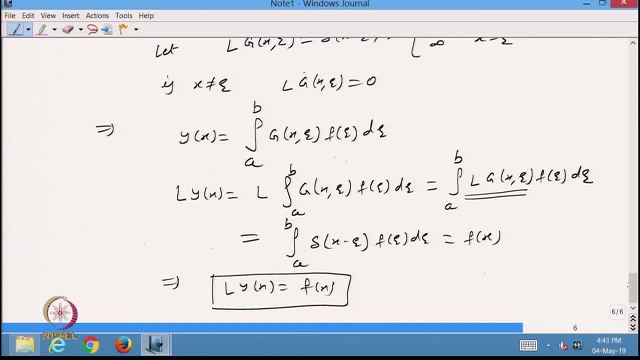 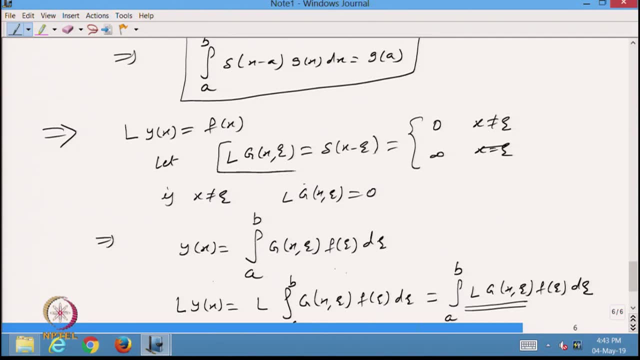 equation we are solving. So from here one thing is clear: that if I, that the we start with this problem, that taking the l, g operating on the Green function, and that is equal to drag delta function, If I apply this one, then my, based on this one, I am able to solve. 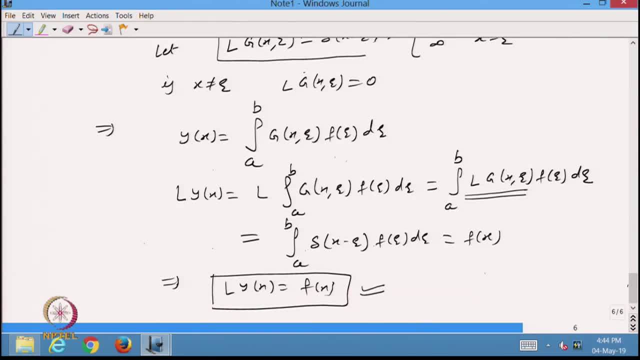 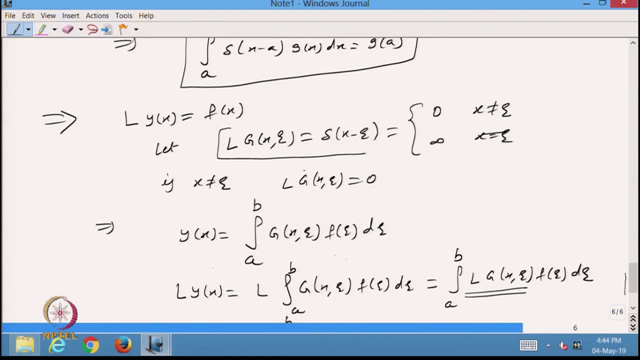 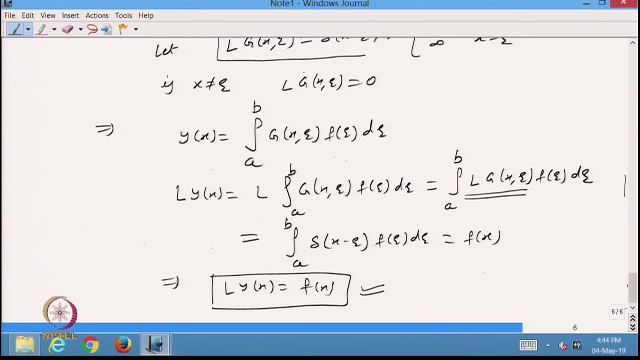 my differential operator or the differential equation. It means that if I am able to solve this equation, then I am able to solve with the help of Green function. I am able to solve this equation And from here I can find out the particular. 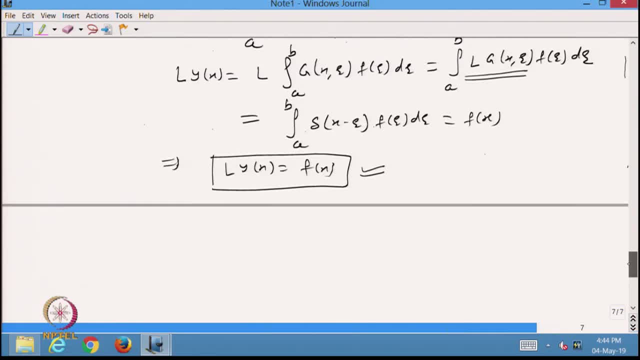 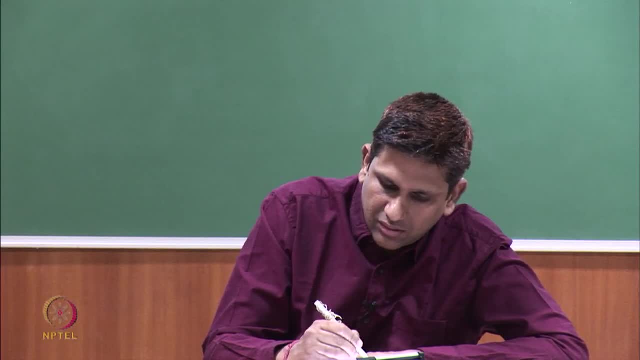 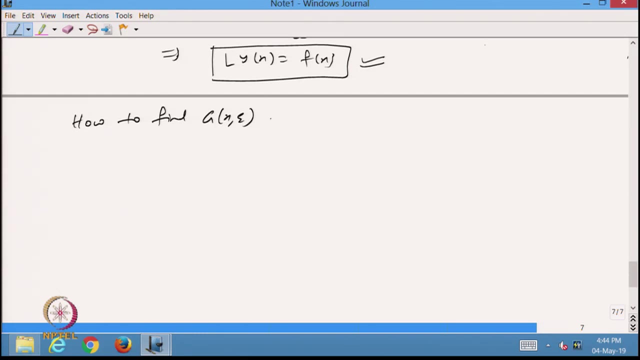 solution of the given equation. Now, the main thing is that now the question is that that how to find that is the Green's function for the given differential operator l. So that is our main goal, that how we can find the Green function. 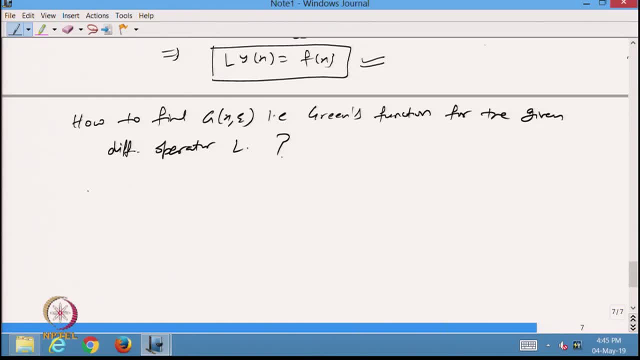 for the given operator. So now you know that my operator l is d square over dx, square plus px, d by dx plus qx. So this one. now what I do is that, if you see that l of applying on the Green function, that is equal. 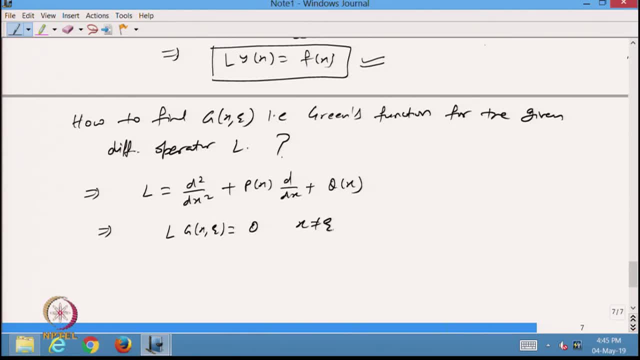 to 0,, basically when x is not equal to xi, because this is equal to drag delta function. So I just want to solve this equation. So this equation, if I want to solve, I know that when x is not equal to xi, it will be 0, otherwise it is infinity. So I want to solve this equation. 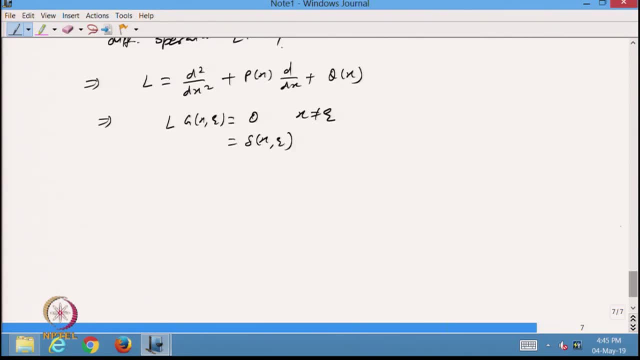 but x is not equal to xi, So let us see what will happen. So if you see this one, so this is the equivalent to the corresponding homogeneous differential equation, And if I am able to solve these differential equation, then I know that from here I will. 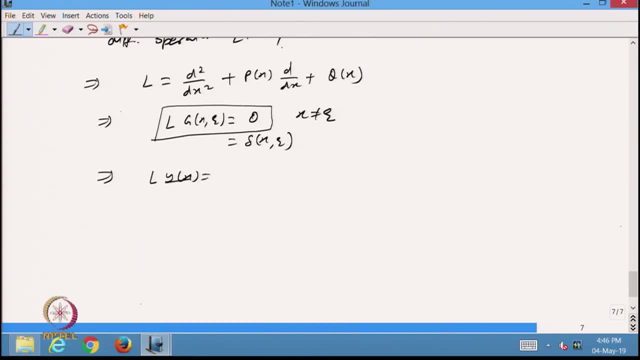 so this equation is equivalent to is equivalent to solving the corresponding homogeneous differential equation for denoted. So this is a solution. Derek, you can use this. why I am not going to use that in the lecture, which is an L start corresponding homogeneous equation And I know that this equation, if I solve, then I 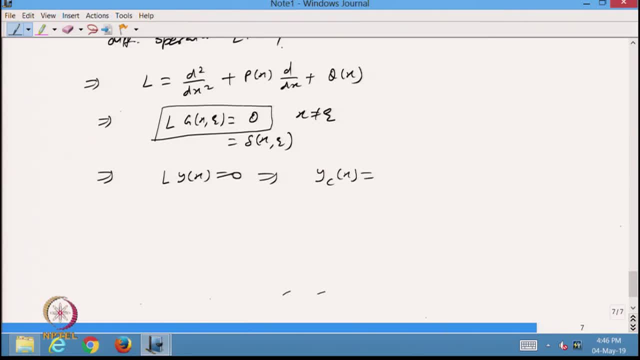 can write the complementary solution of this equation. If I am able to find two linearly independent solution and I can write that the c1- y1 x plus c2 y2 x, So this, I am able to do this one. So once we are able to find this value, so based on this one, I can define 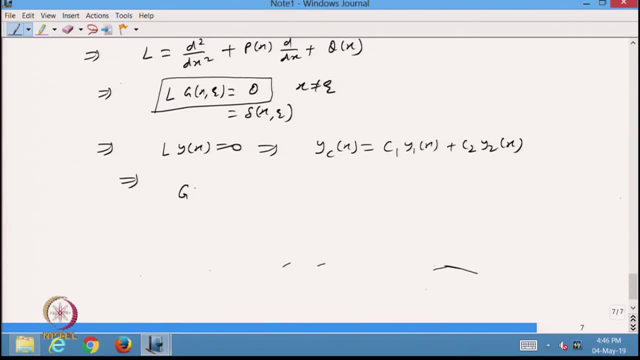 my green function. So in this case I just define my green function. So this will be: I just define c1- y1 x plus c2 y2 x. So this is because x is not equal to xi. So in this, 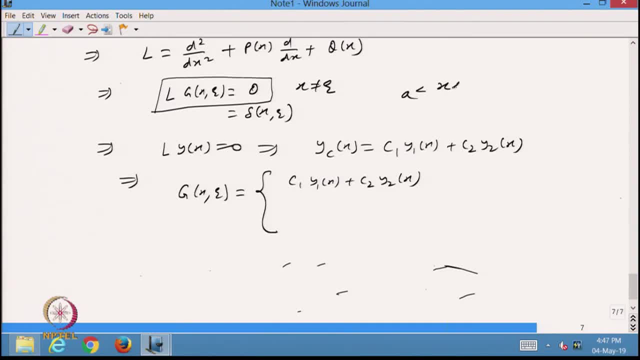 case I am taking, my x is lying between a and b, So xi is also lying between a and b. So this one, I can say that this is when x is less than xi. And another one I take d1- y1 x plus d2 y2 x, And this is the case when x is greater than xi, Because x equal to xi. 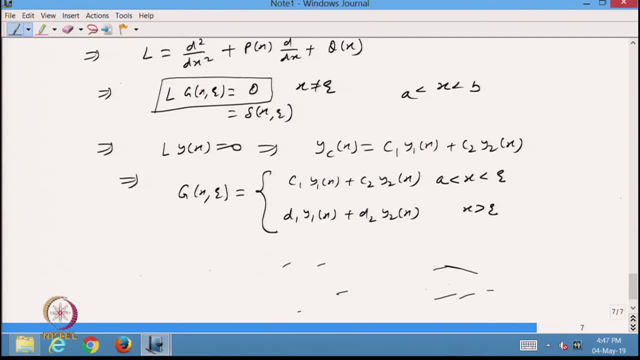 this will be infinity, so that we are not interested. So this is the corresponding green function we are able to define. Now the question is that that I am able to define my green function, So I have c1, c2 and d1, d2, these are the 4 constants we need to find out to define. 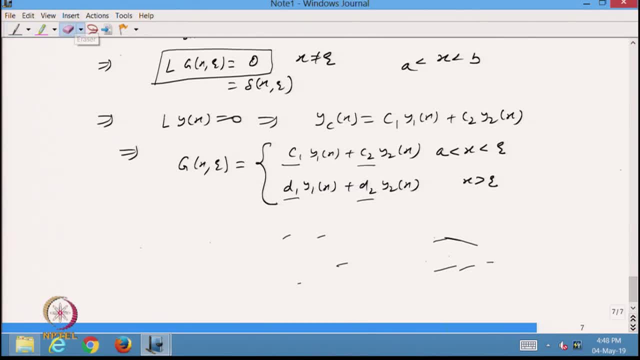 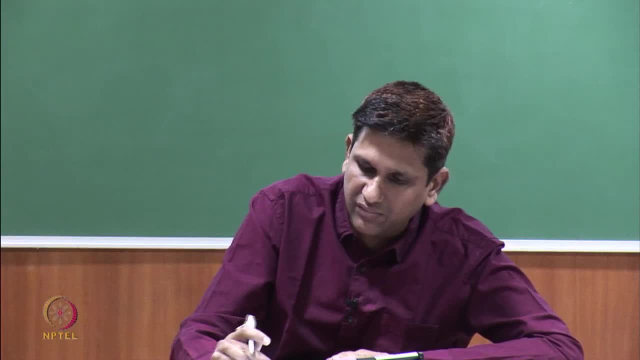 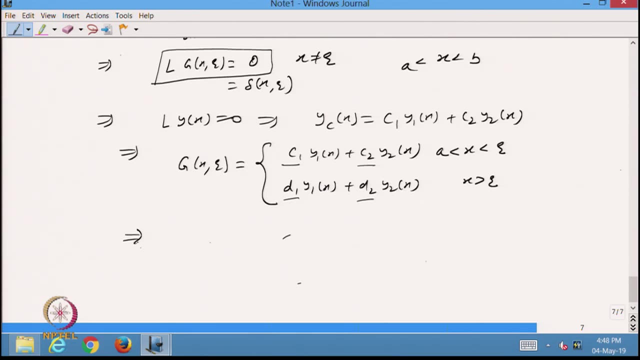 the given green function. So this one we can define with the help of the following properties of the green function. So from here the properties we are going to use for find out this interval. So let us do this. So here we have the following properties: 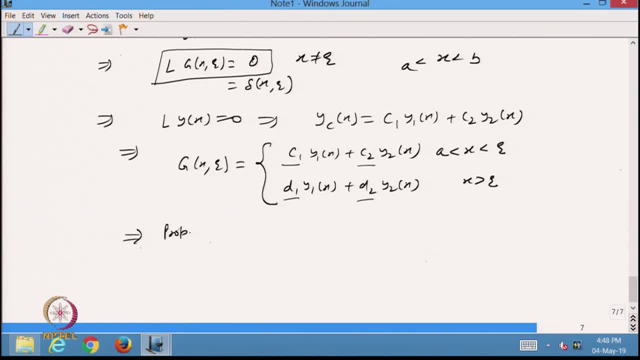 out this interval. the first property is: so this is the properties. The first one is that the green function g, x, xi is continuous at x equal to xi. So in this case, if this is a continuous at x equal to xi, So from here I can say that the c1- y1 xi plus c2- y2 xi. 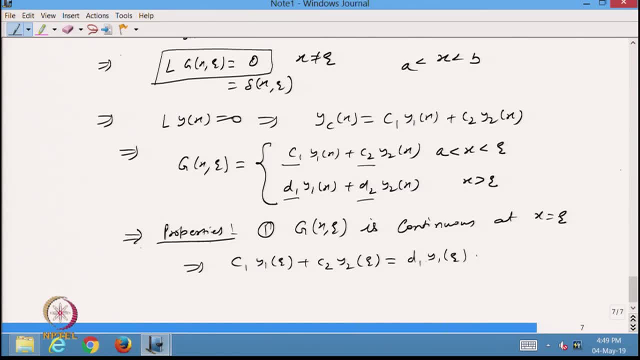 is equal to d1 y1 xi plus d2 y2 xi. And from here I can say that c1 minus d1 plus d2 y2 xi, y1 xi plus c2 minus d2 y2 xi, that is equal to 0.. So this is the first equation. 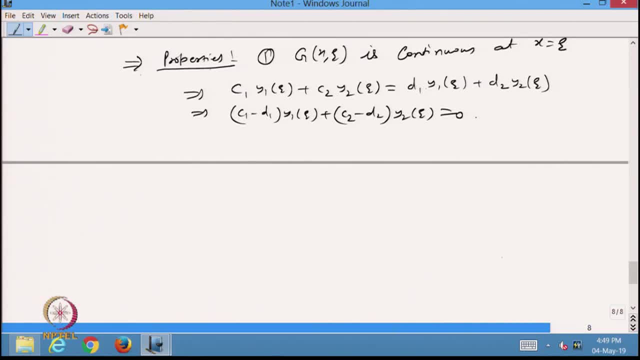 we are dealing with. So this, I call it equation number 2.. So this is the first property. The second property is that second property is that that del g by del x has, del x is a jump discontinuity of magnitude 1, at x equal to, at x equal to xi. 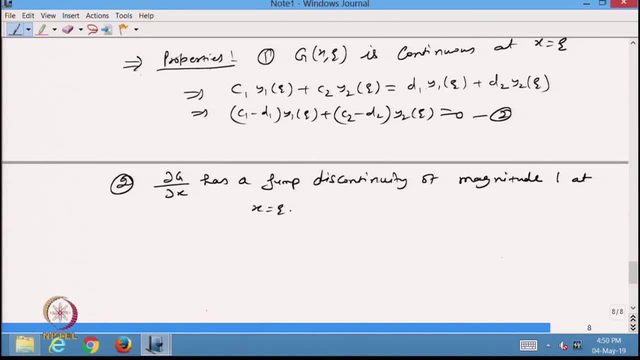 So these are another property. So if you see, from here I can, from here I can define that del g over del x, for x greater than xi, minus del g by del x, x less than xi. So this is defined at x equal to xi. So this is equal to 1.. So from here we can say that. 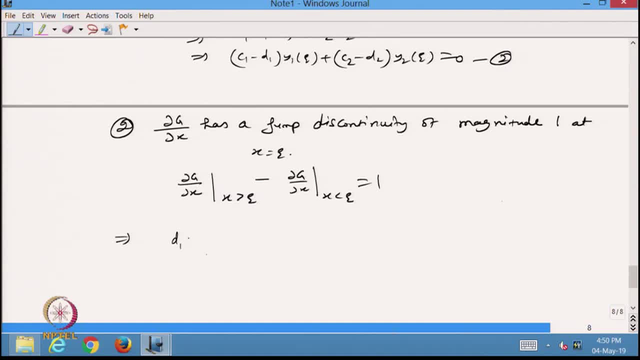 that d1 y1 xi plus d2 y2 xi minus c1 y1 xi, c2 y2 xi, that is equal to 1.. So from here I can say that that d1 y1 xi minus c2 y2 xi, that is equal to 1.. So from here I can. say that that d1 y1 xi plus d2 y2 xi, that is equal to 1.. So from here I can say that that d1 y1 xi minus c2 y2 xi, that is equal to 1.. So from here I can say that that d1. 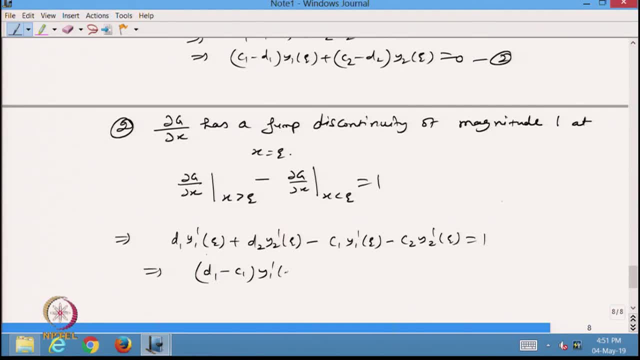 d 1 minus c 1 y 1 xi, plus d 2 minus c 2 y 2 xi, that is equal to 1.. So this is another equation we are going to have. So this is equation number 3.. So now you can see that. 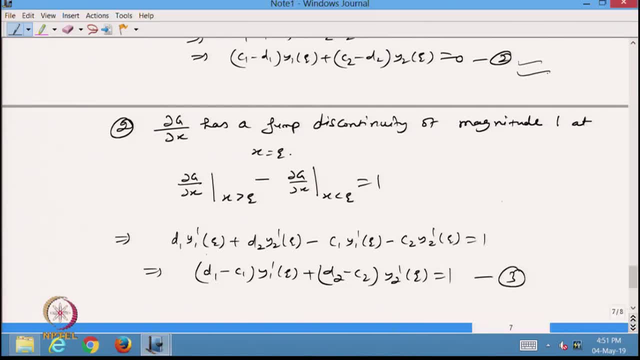 I have equation number 2 and this is the equation number 3.. So we have 2 equations and we have 4 variable. 4 variable: c, 1 c, 2 d, 1 d, d, 1 d, 2.. So that we have to find out. 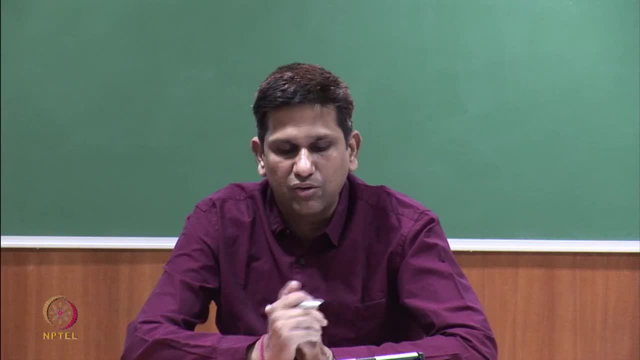 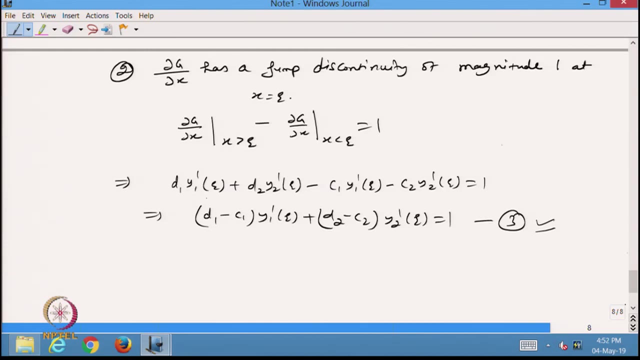 So in this case I need 2 more equation to find out the value of all the c 1 c, 2 d, 1 d, 2.. So that values basically. so those values are those conditions I needed. So 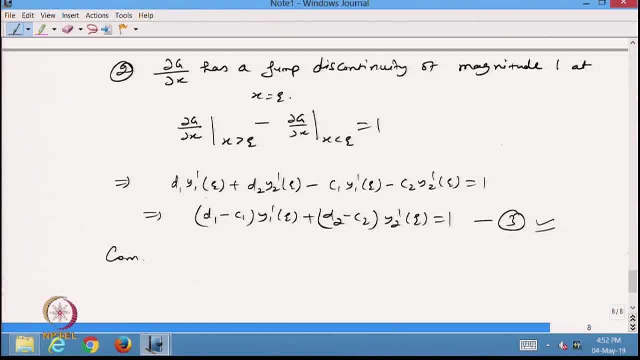 those condition will come from. So those condition will be coming from either. you know the initial value problem, that is, we have some y at x naught equal to 0 and y dash at x, naught equal to 0.. So this is the initial problem I am defining, or I will define the. 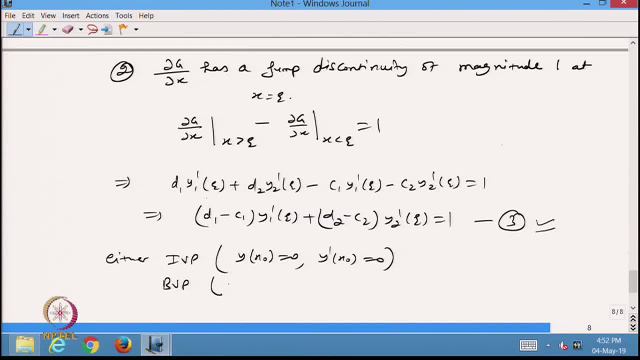 boundary value problem. So boundary value problem I will define: like y at x, naught is equal to so some value that I call it alpha, and y at some x1, that is beta. So this also I can define. it may not be 0 always, it can be known 0 also. So I just define this as 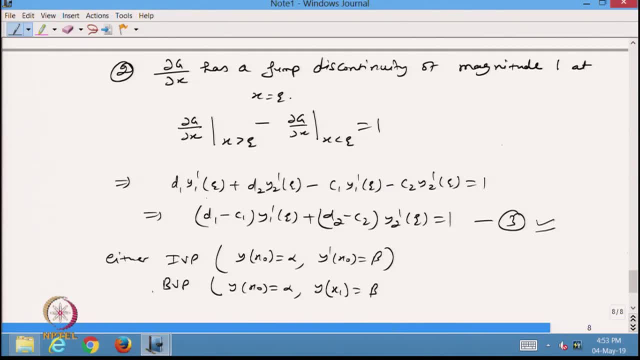 a, also alpha, and this is equal to beta. So this is my boundary value problem and this is my initial value problem. So this is my boundary value problem and this is my initial value problem. So if I solving the initial value problem and try to find the green function, 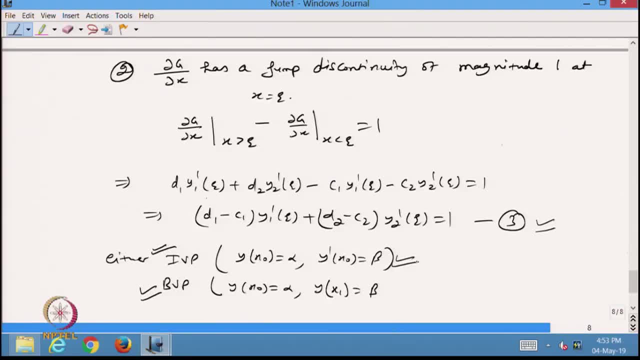 for the initial value problem, then I will take the help of this one, and if I am solving the boundary value problem, then I will take the help of this one. So, based on this one, we will able to get two more condition and after having the four, 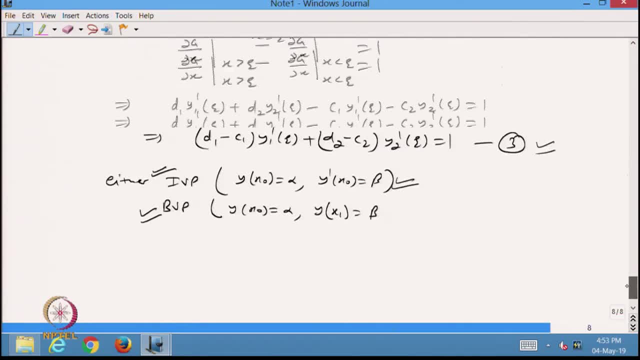 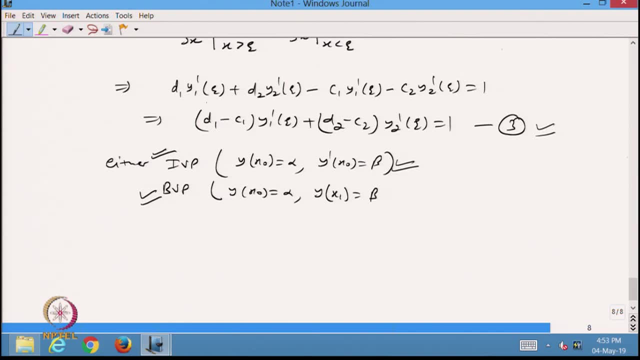 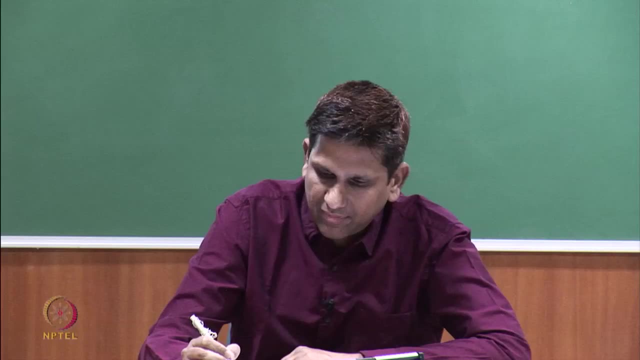 condition, that is, equation number 2, equation number 3 and the two condition. from here we are able to find out all the value of c1, c2, d1, d2, and then we are able to define the green function for the given linear differential operator. 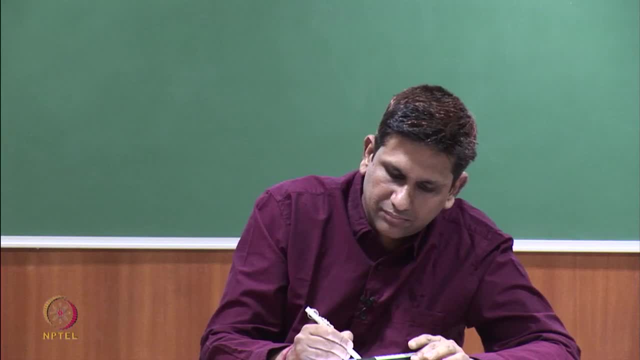 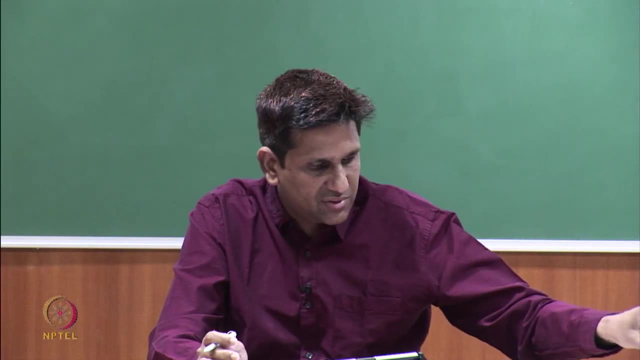 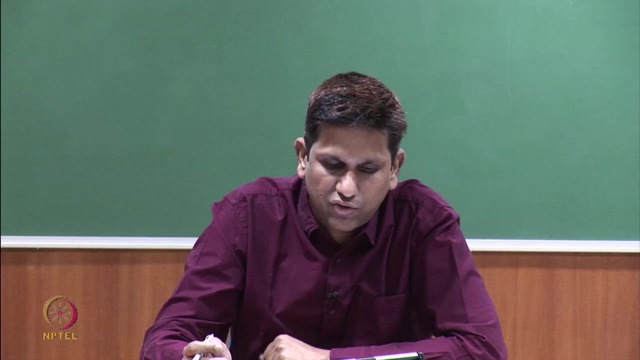 So now. so let us define, let us do one example of based on this one, because if you see, then the same thing we have done for you with the help of variation of parameter also, So in this case also I can find out. 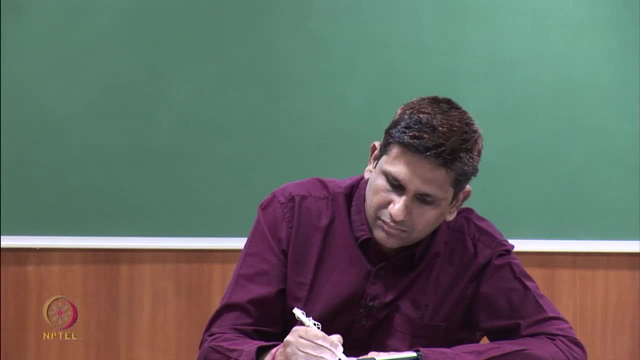 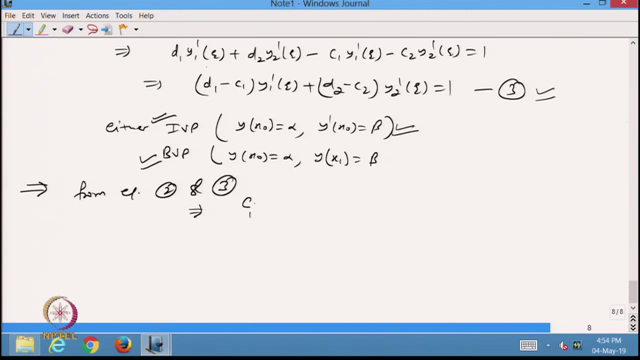 So from here, so from equation number 2, 2 and 3, c1 minus d1, this is y1 x. So I just call it y1, because we have to write c2 minus d2, y2.. that is equal to 0, and then I have defining this one. So this is again I am defining. 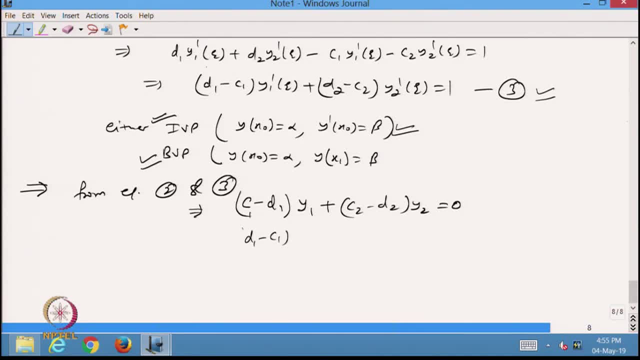 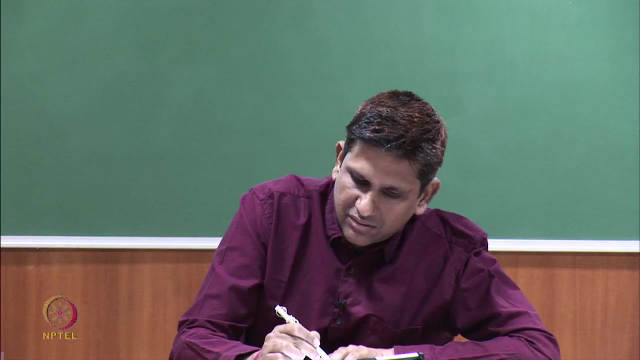 so that will be d1 minus c1 y1 dash plus d2 minus c2 y2 dash is equal to 1.. So from here I can define. so this one I just because this value, if you see. so this one I just I can. 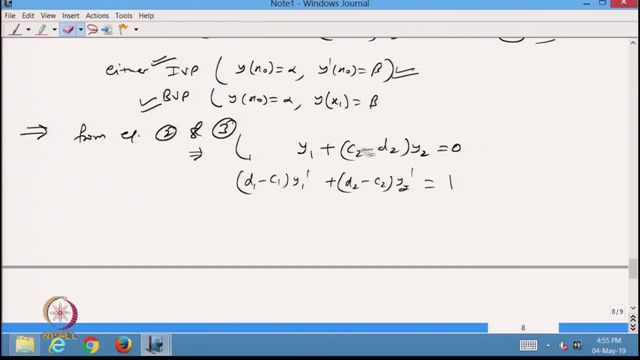 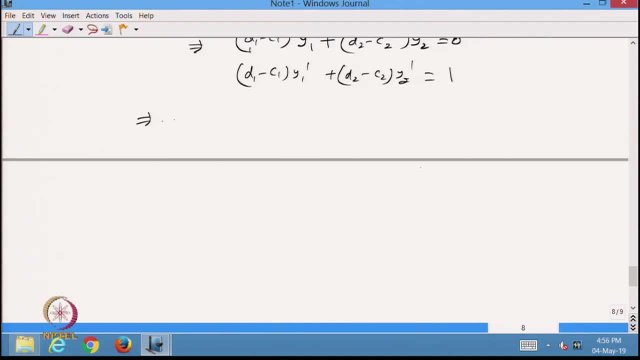 write this function also like this one, just changing the position of, so I can write this as d1 minus c1 and d2 minus c2.. Okay, So now I have a two equation. now I know that. so from here I know that my y1 x and y2 x 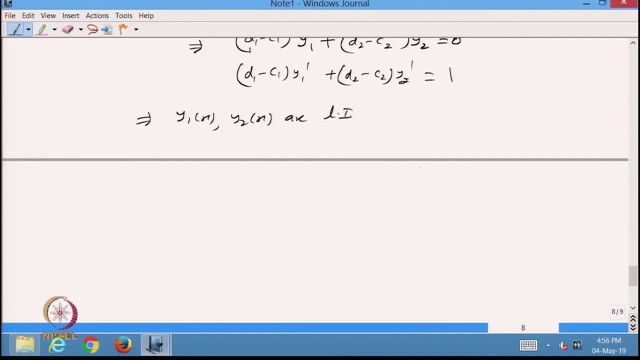 are linearly independent. So if they are the linearly independent, then I know that the corresponding Wronskian. So this Wronskian we have defined. So this one, y1 and y2, x, will be not equal to 0. So in this case, if this is not equal to 0, then this will be. 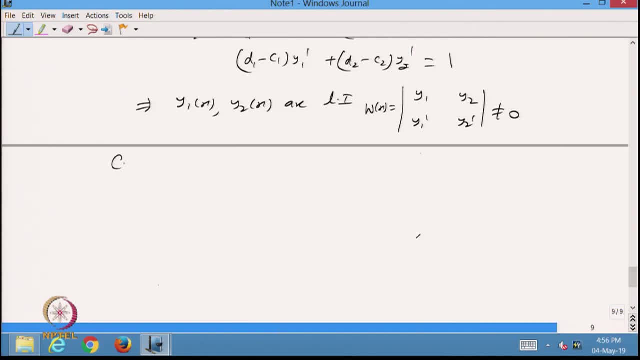 linearly independent and with the help of the Cramer's rule, I can find the solution of this one. So though, that solution if you, if I find out, So this one will be Okay. So we have already done this one. So d1 minus c1, I can define, So this will be equal. 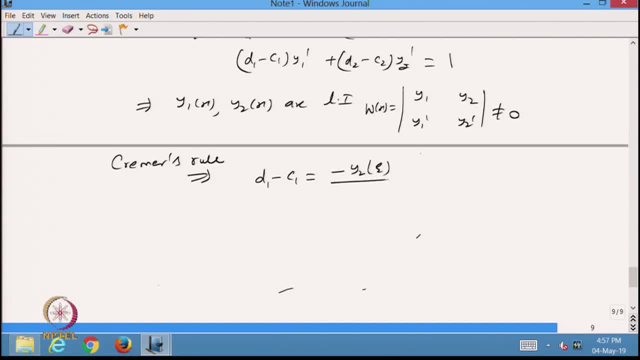 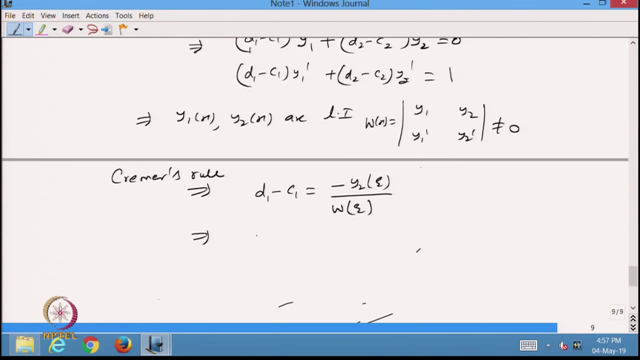 to minus y2 over the Wronskian, at this one x equal to xi. So this one I already know. and from here another equation: if I want to write, then d2 minus c2 will be y1, xi over the Wronskian at x equal to xi. So this is the value of the coefficients, value of the. 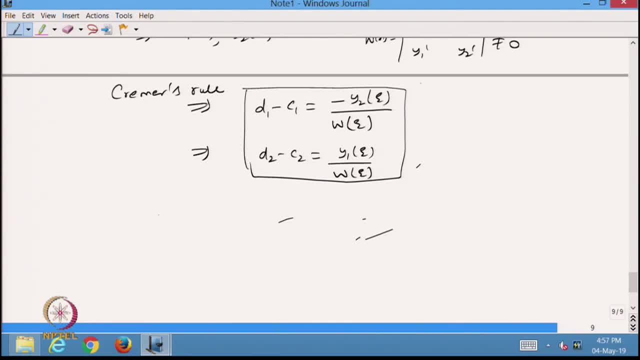 variable d1 minus c1 and d2 minus c2, that we already we have done for the when we will taking doing the variation of parameter. So with the help of this one Now, I can define now the. so from here, now, in this case, I can assume that this: 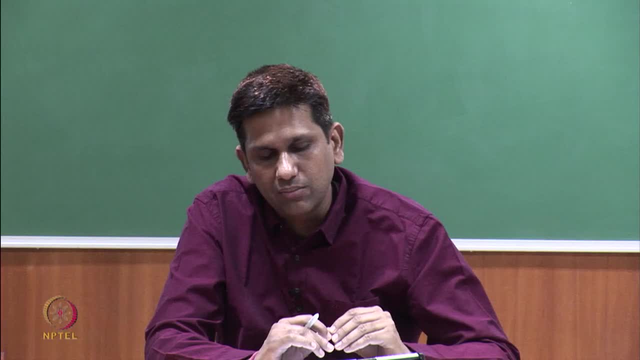 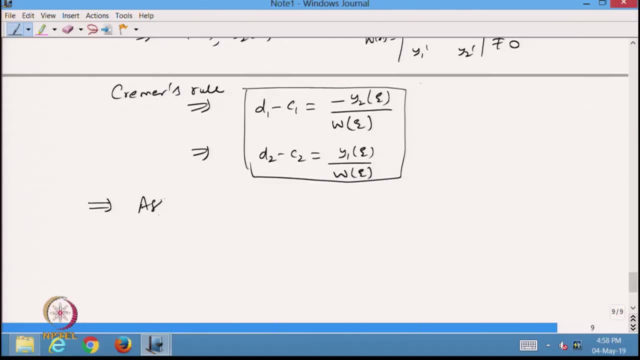 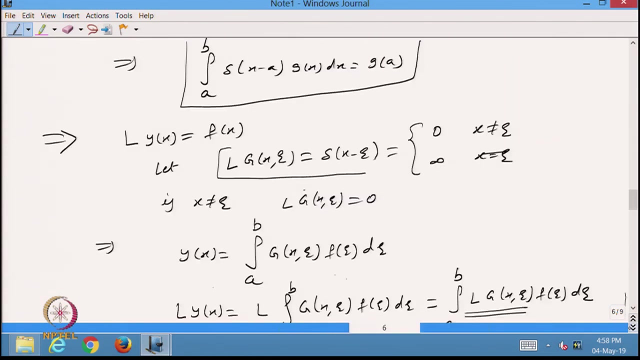 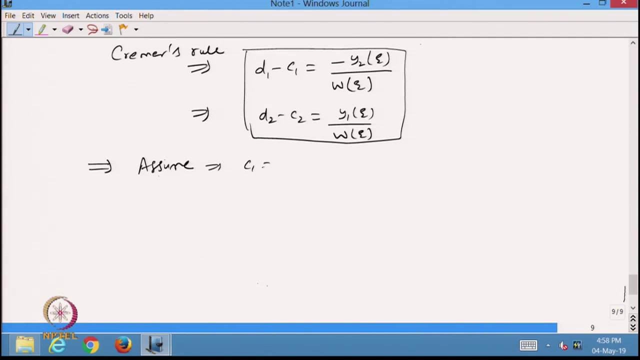 condition is either initial problem or the boundary value problem. So just in this case, I assume that. assume that that let we are assuming Then by now we are assuming that my c1 and c2, they are 0. So let us assume that. 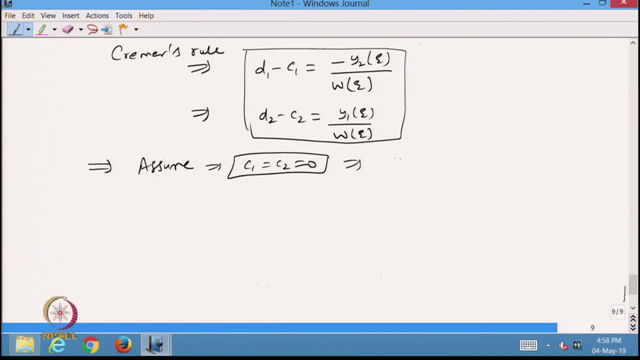 one. So in this case, if I'm assuming this one, then I can say my d1 will be minus y2 xi over Wronskian and d2 will be y1 xi and that is Wronskian. Now Tarlyios question. 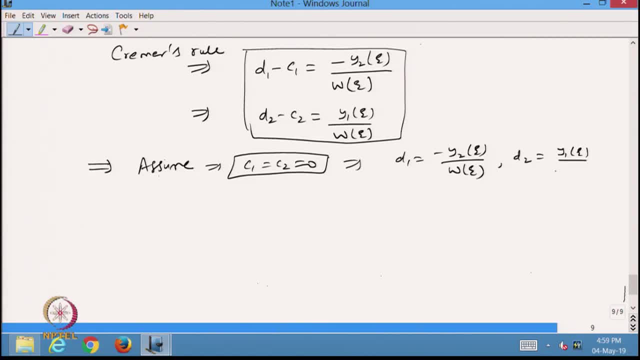 is one thing, And then what I can do is this: I can say this: This is the one thing that can be defined. So donation, All these Right, It is not to tell you what it is, I will just express for you. But when? 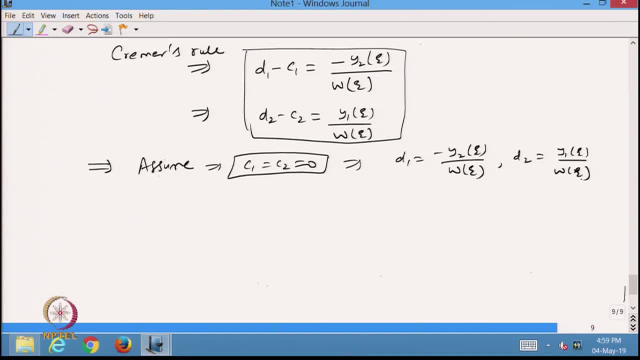 I can say that, Yes, I can crab a problem over there, but I will. yes, I can say: that is fine, that at this point. So from here I can define my green function as xi. So I have taken. 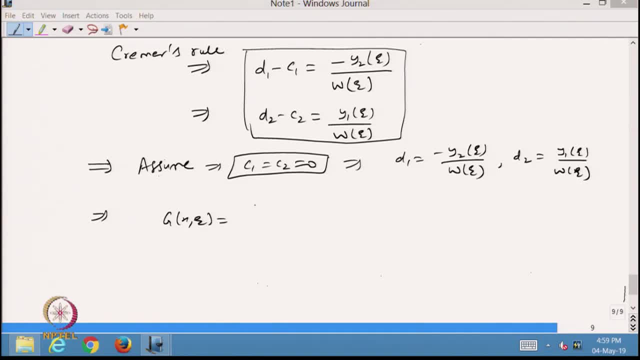 my c1 and c2 equal to 0. just I am taking this one, So in that case this will be: is equal to 0 when x is less than xi, and this will be equal to minus y2 xi y1, x, plus y1 xi- y2. 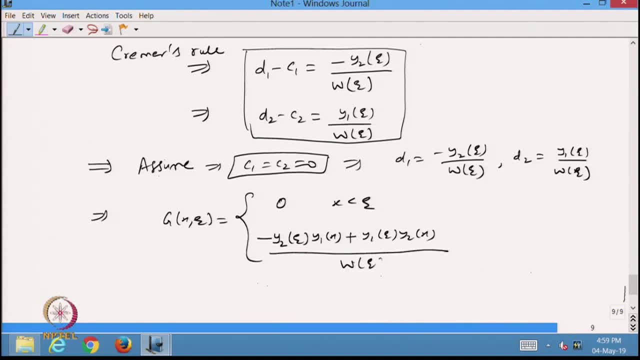 x divided by the Wronskian, when x is greater than xi. So from here I can say that this will be equal to 0 when x is less than xi. and this will I can define as y1 xi, y2 x minus y2 xi, y1 x when x is greater than xi. So this is: 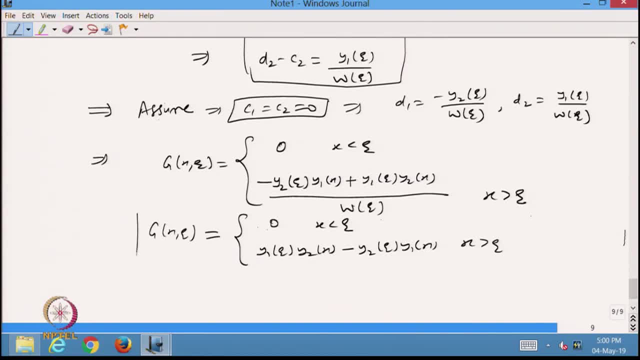 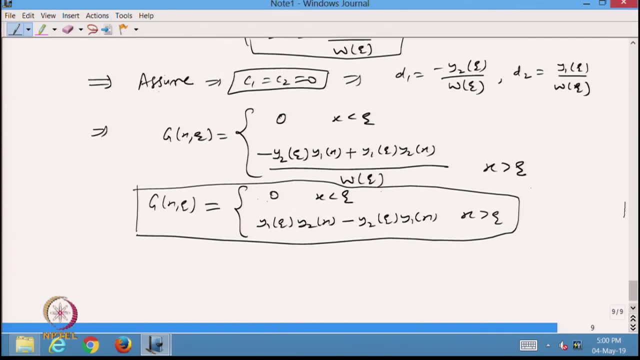 my green function. So in this case we can, because I know that I am also solving this equation. So this equation basically 0 when x is not equal to xi. So this equation does not have a unique solution, Because if I have g, x, xi is one of the solution. 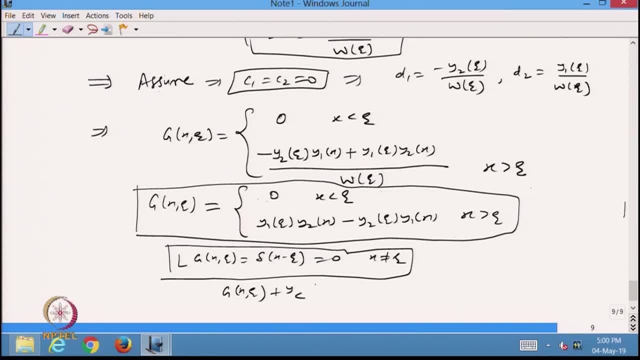 then g x, xi plus yc. that is the complement solution. that is again the solution of this equation. So this equation does not have a unique solution. So in this case, g x, y, depending on that, I have chosen, in this case c 1 and c 2, equal to 0, I got this Green function, If I have. 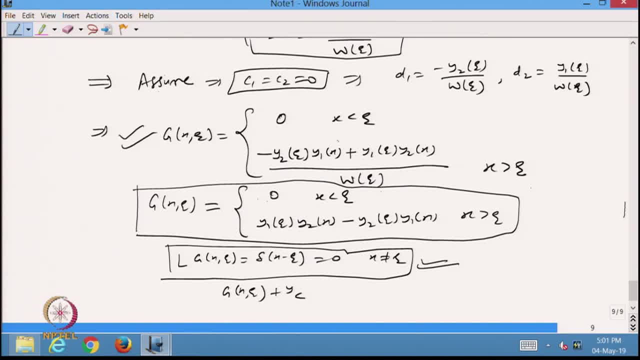 chosen c 1 equal to 0 and d 1 equal to 0, then this Green function would have been the another one. We have to choose c 1 equal to 0 and d 2 equal to 0, then we get the another.